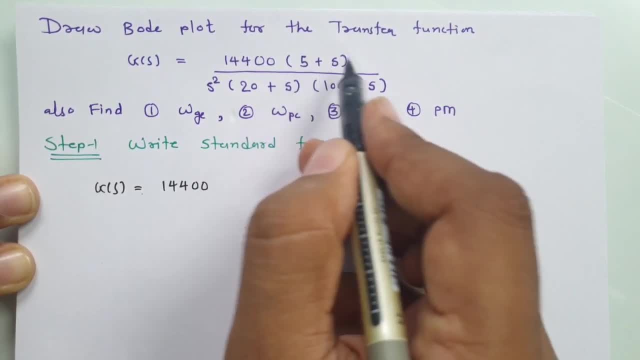 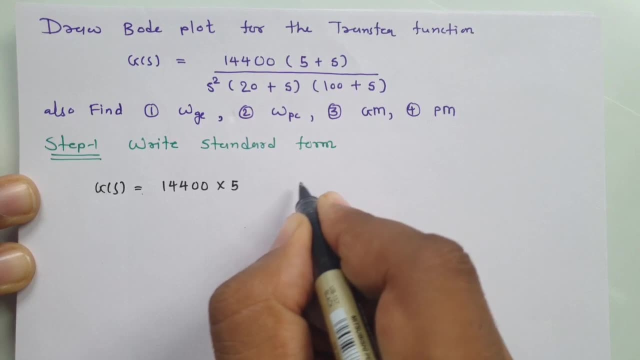 here you see, phi plus s. that is there in numerator. So I need to take phi common from numerator And here I'm writing this: poles and zeros in standard form. So I need to say one plus s by phi right Now in denominator. see, this is s square. So that is as it is. 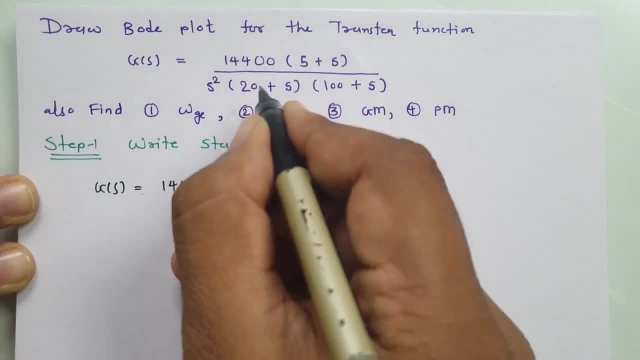 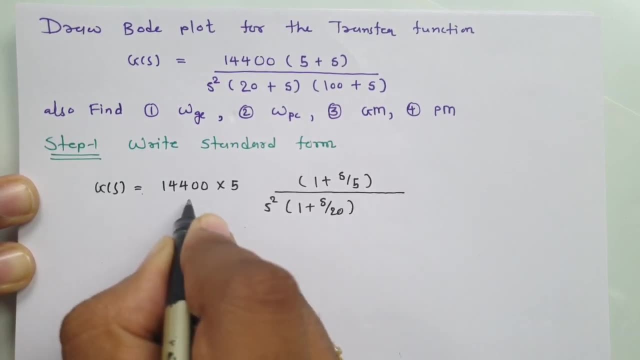 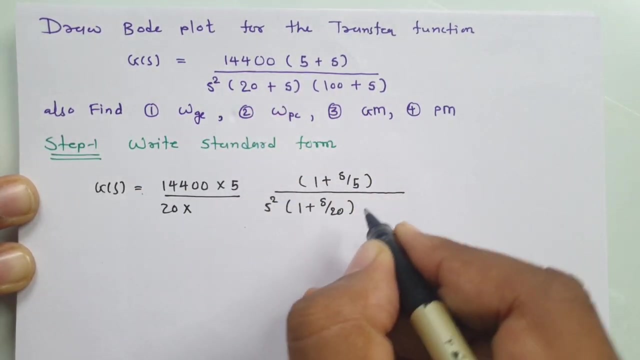 And now you see 20 plus s is there, So I need to take 20 common from this. So this will be one plus s divided by 20.. So here I need to write 20 in denominator, as I have to 20 common. and here 100 plus s is there, so I need to write one plus s by 100 by taking 100 common. 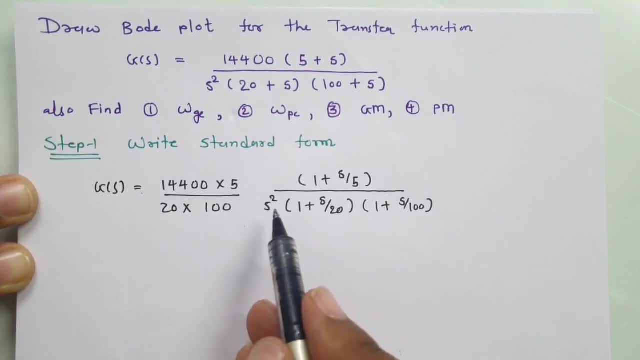 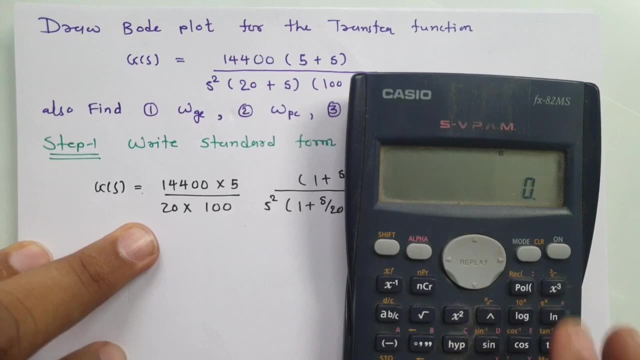 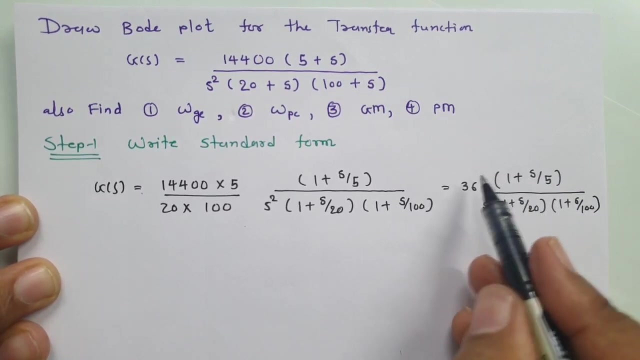 So here I am taking 100 common like this. So this is how I need to write standard form. Now let us write this value of constant: So that is 36.. So this is our standard form Right Now. next step is to identify slope of first line. 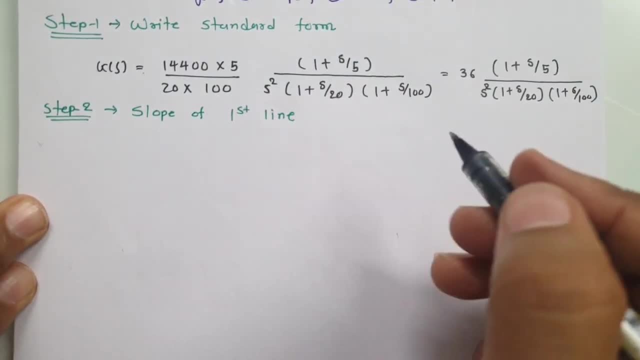 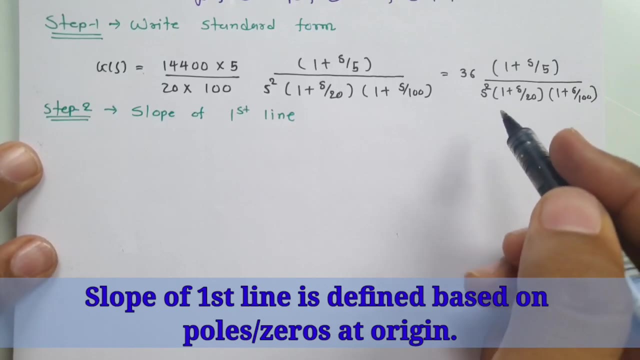 Now see, I have told you already in last video slope of first line that is based on poles and zeros at origin. And if you observe this transfer function, then at origin there is two poles. Right, You see, in denominator there is s square means. there are two poles at origin means. 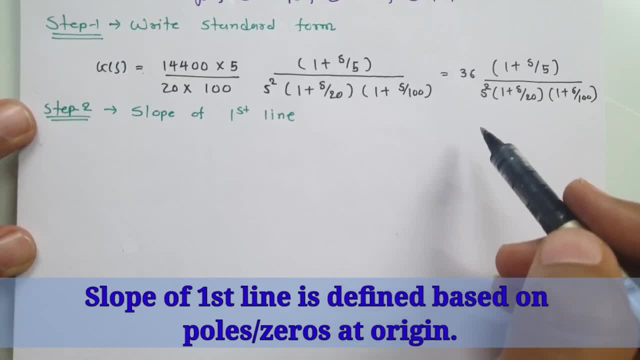 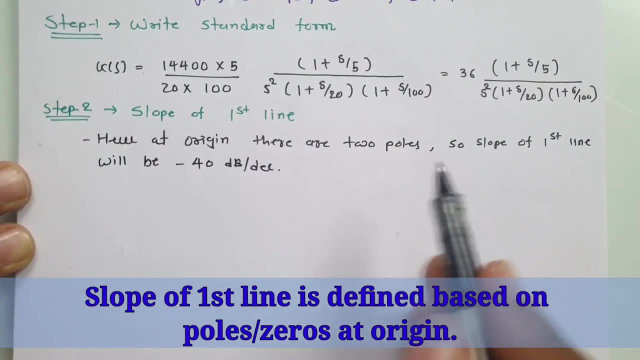 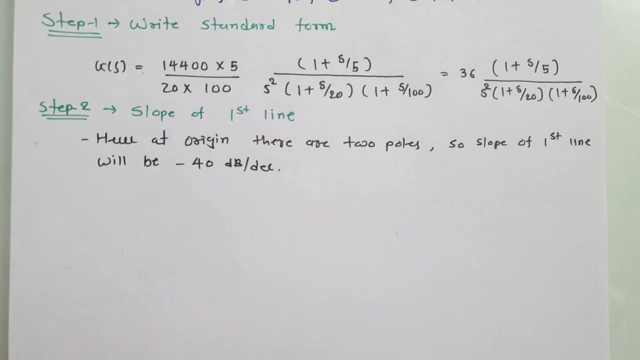 slope of first line will be minus 40 dB per decade. So slope of first line that will be minus 40 dB per decade. Now next step is to identify gain of first line at omega is equals to 1 radian per second. 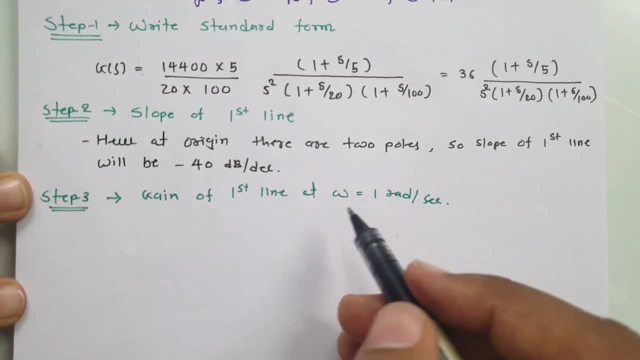 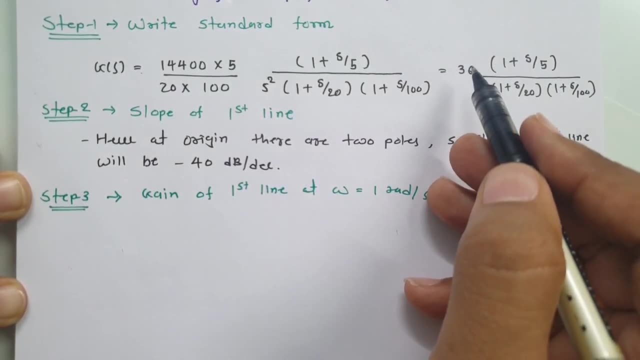 So gain of first line at omega is equals to 1 radian per second. That is based on standard form. Now you see, in standard form we have constant that is 36.. So already we have calculated constant k, that is equals to 36.. 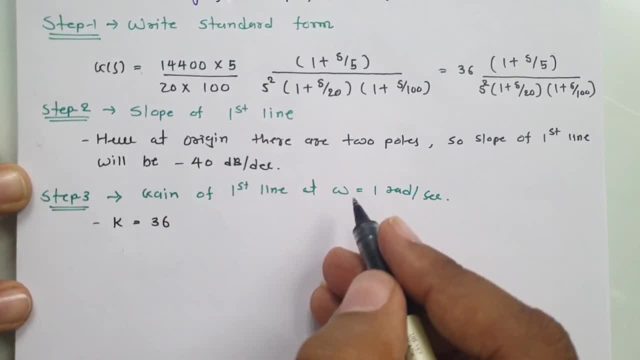 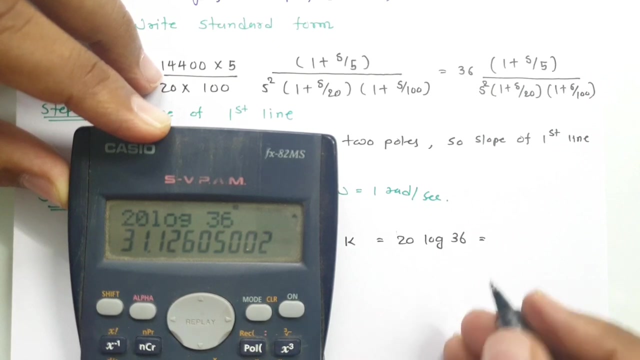 Now, based on this, we can have gain of first line at. omega is equals to 1 radian per second And that is 20 log of k. here k is 36. So 20 log of 36. And if you solve this, so that is 31.12.. 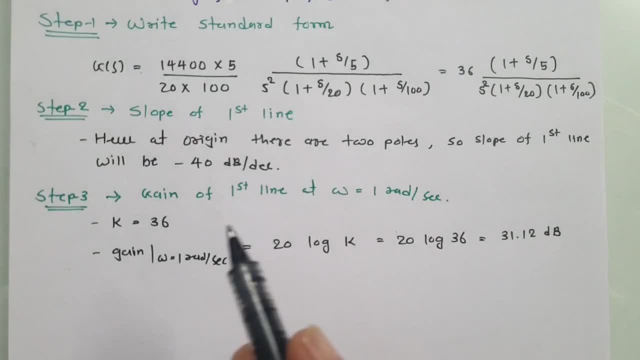 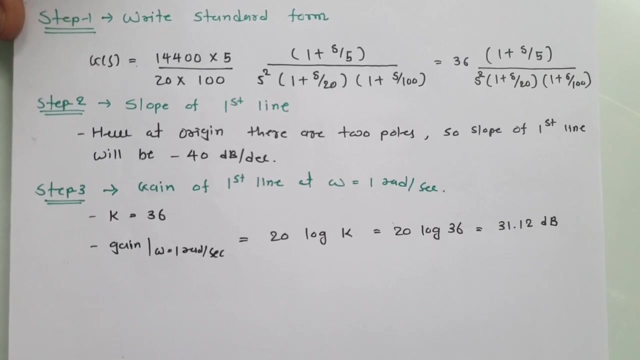 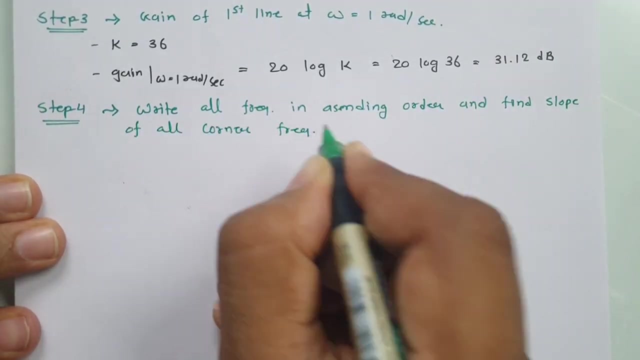 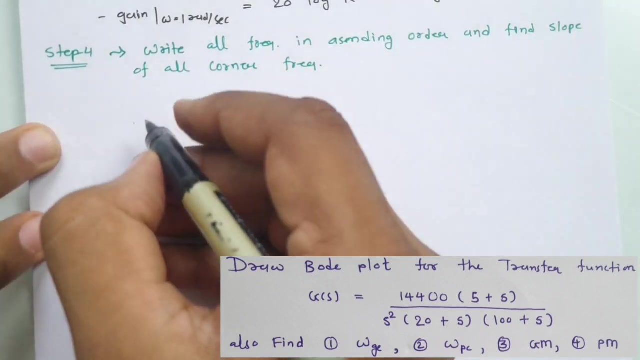 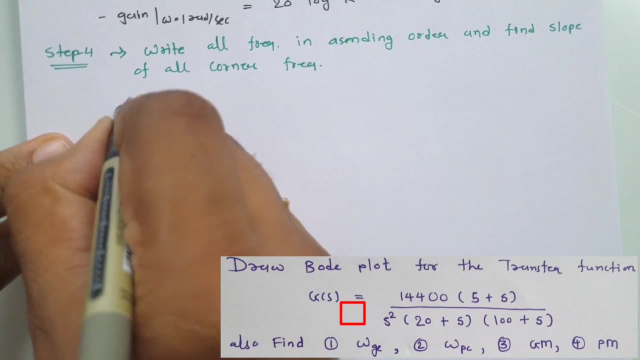 So gain of first line at omega is equals to 1 radian per second, That is, 31.12.. Now next step is to write all the frequencies in ascending order And we need to identify slope of each corner frequencies. So if you observe our transfer function, then here we have. corner frequencies at origin means 0. 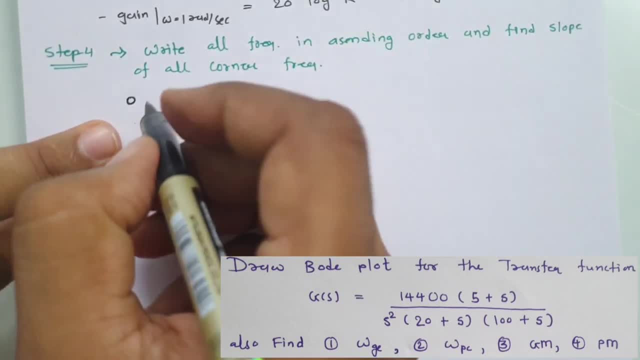 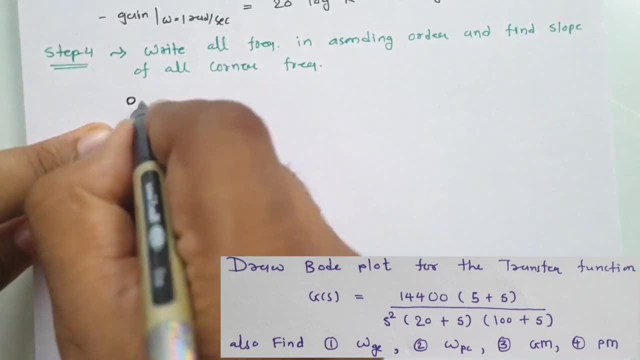 So after that, if you see, corner frequencies are 5.. 20. And 100.. Right, So here we have corner frequencies like this: 0 is lower than 5.. Is lower than 20.. Is lower than 100.. 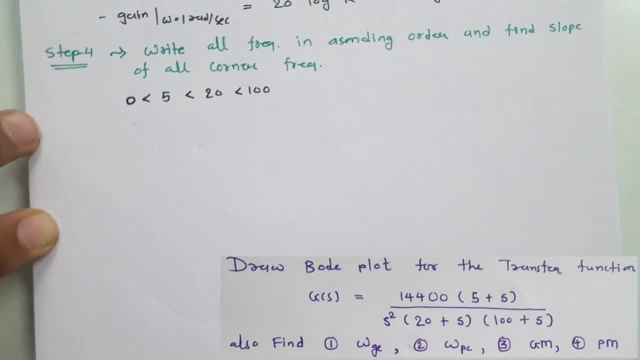 See, this is how corner frequencies are there with us. So I need to write all the corner frequencies in ascending order. Now I need to mention pole or zero, which is there with this corner frequency. so at origin we have two poles, right? so i need to say here we have pole, and in bracket i am writing: two poles are there. 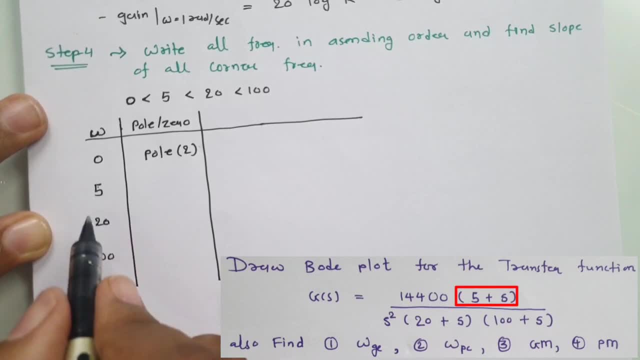 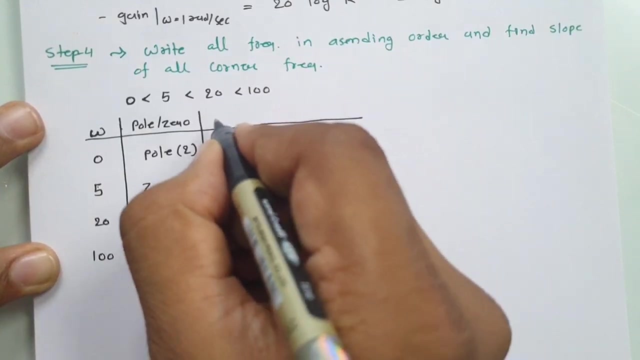 now, you see, at phi corner frequency we have zero. so here i need to say there is zero. now, at 20 there is pole, so i need to say there is pole. at 100, there is pole, so i need to say there is pole. now, here i will be writing slope. 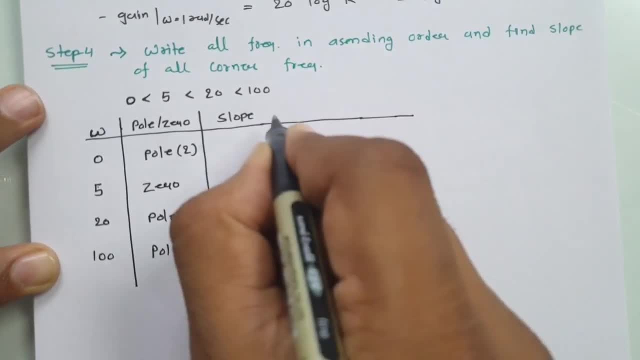 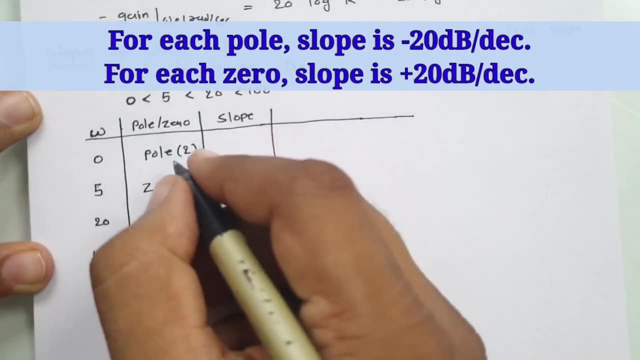 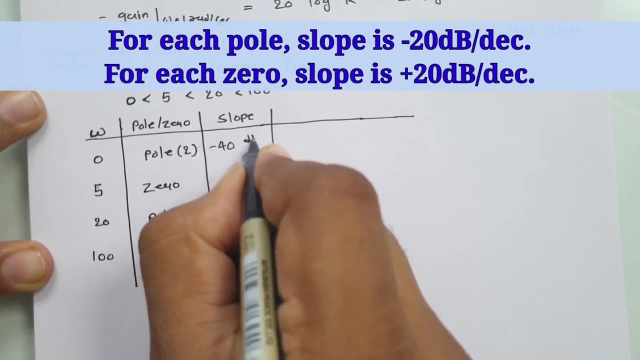 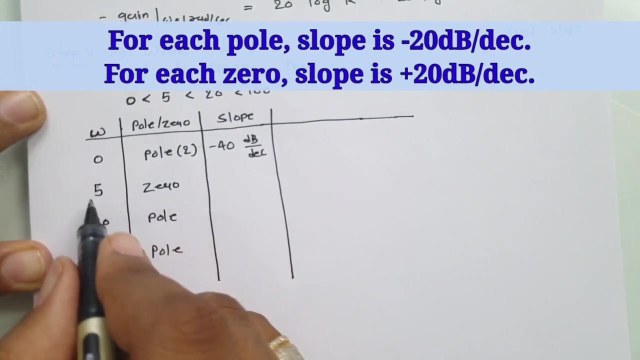 for each line and then we will identify resultant slope right. so see, at origin there are two poles. so for one pole slope is minus 22 dB per decade. So for two poles slope will be minus 40 dB per decade. Now there is one zero at five, So slope will be plus 20 dB per decade for one zero. Here there is one. 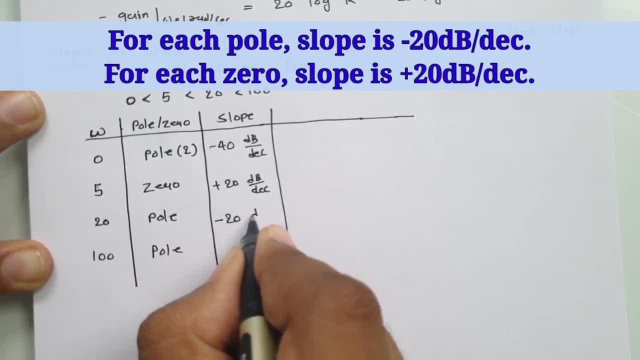 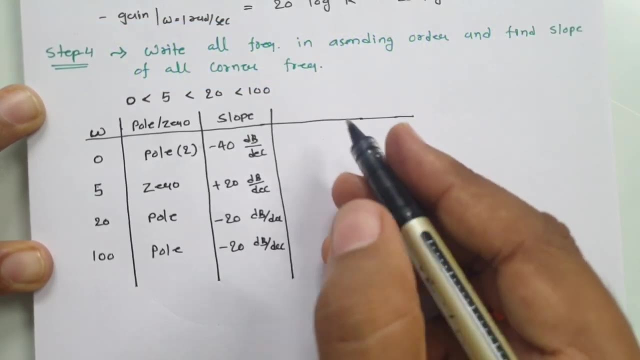 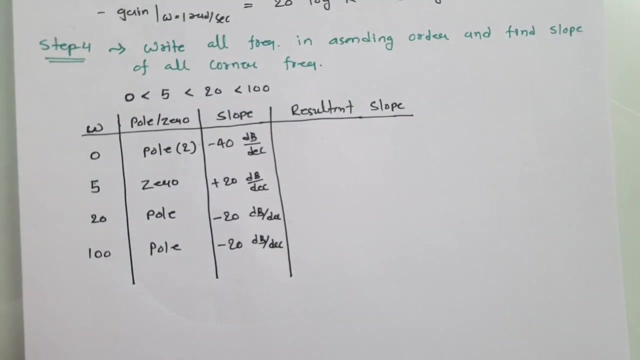 pole at 20. So slope will be minus 20 dB per decade for one pole. And here at 100 there is pole, So slope will be minus 20 dB per decade for one pole. Now here we will calculate resultant slope. So to calculate resultant slope, see first line is having slope which 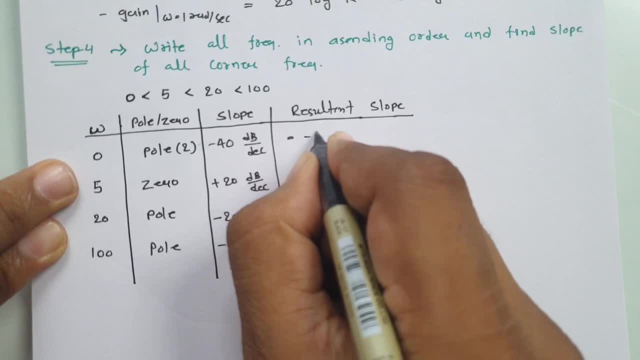 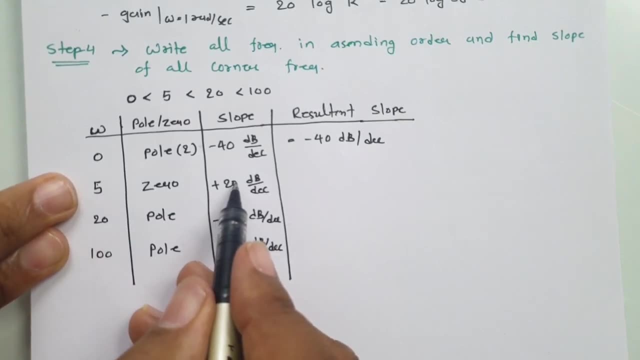 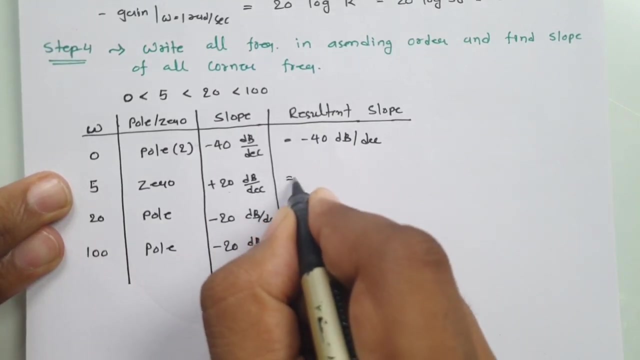 is minus 40 dB per decade. So I need to say slope is minus 40 dB per decade. Now next corner frequency is having slope plus 20 dB. So previous plus current, So minus 40 plus 20.. So here slope will be minus 20 dB per decade. 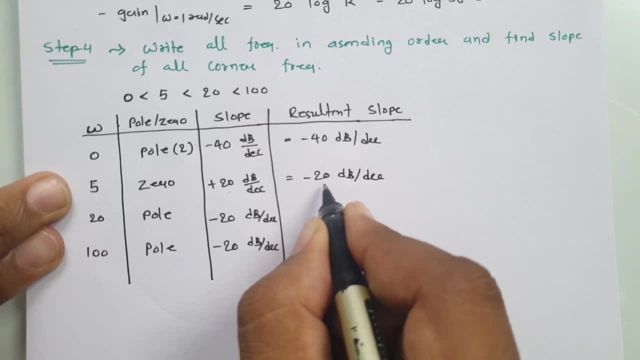 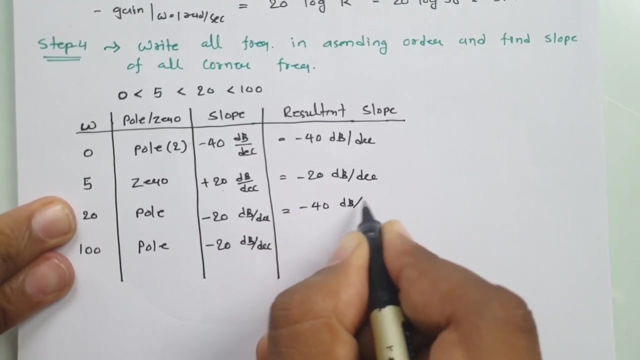 So resultant slope of second corner frequency that is minus 20 dB per decade. Now see here: with this corner frequency, previous slope is minus 20, current is minus 20.. So minus 20, minus 20, minus 40 dB per decade. And then 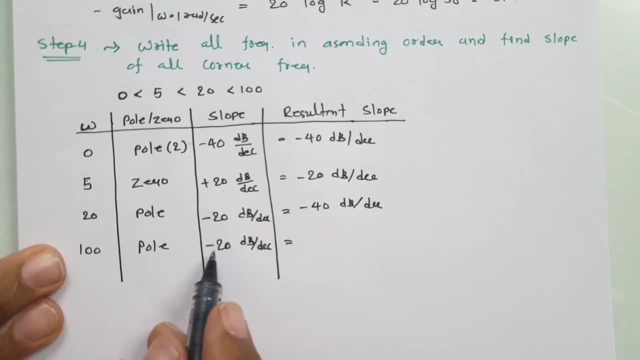 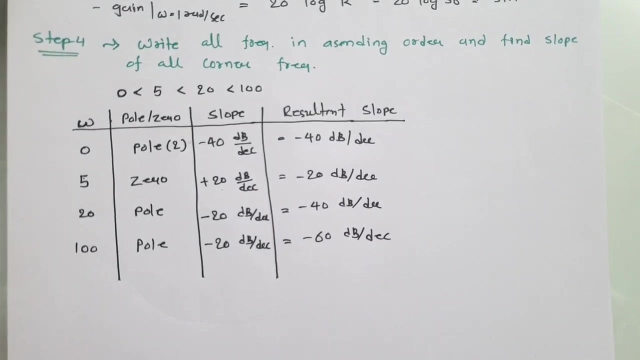 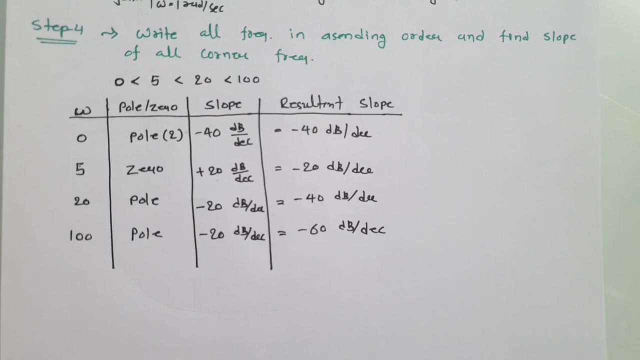 at 100 corner frequency there is pole, so that is having slope minus 20 dB per decade. Previous is minus 40. So minus 40 minus 20, that is minus 60 dB per decade. So that is how we can have resultant slope of each corner frequency. Now step number five, that is, to write given. 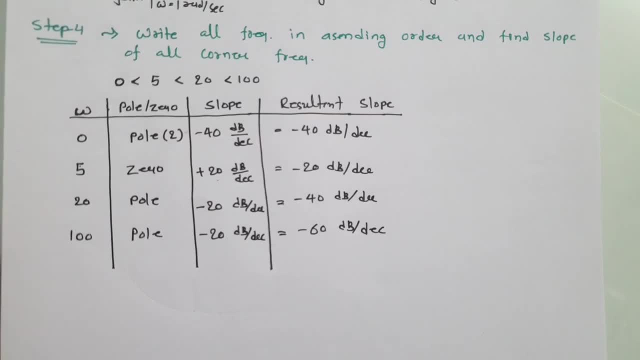 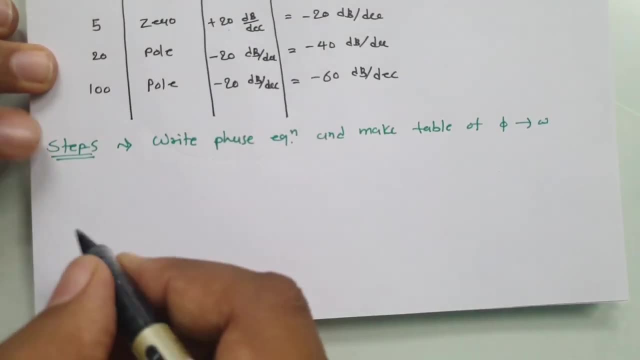 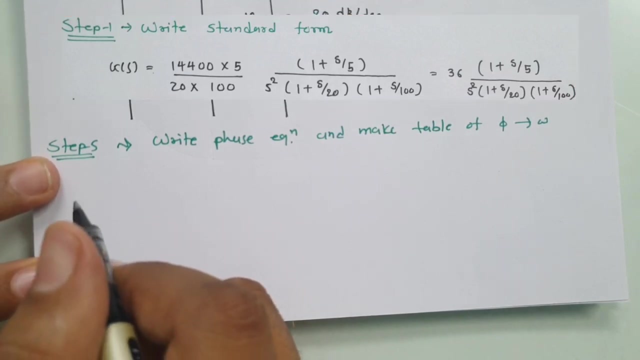 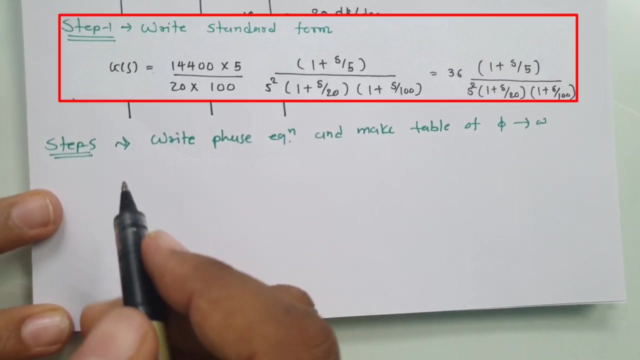 systems phase equation. Then we will make a table of phase with respect to frequency. So if you observe our transfer function, then in the transfer function we need to place S equals to j, omega right, And we need to write phase equation. Now you see, at origin there are two poles. So here Pepper. 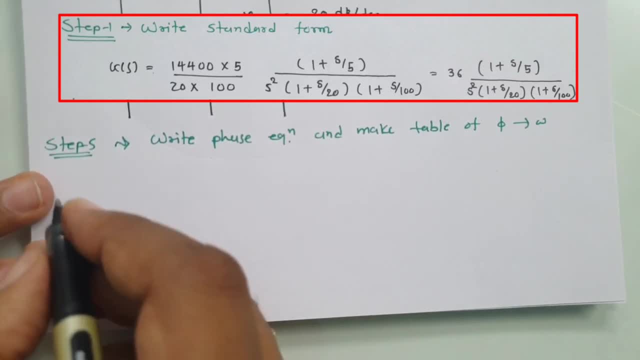 tilde is equal to J omega, and here Episode Víi, that will be H É Newton nãoNé. so here for those two poles. one pole is having minus 90 degree phase at origin, so two pole is having minus 180 degree phase at origin. then you see, there is one zero at omega is equals to five. 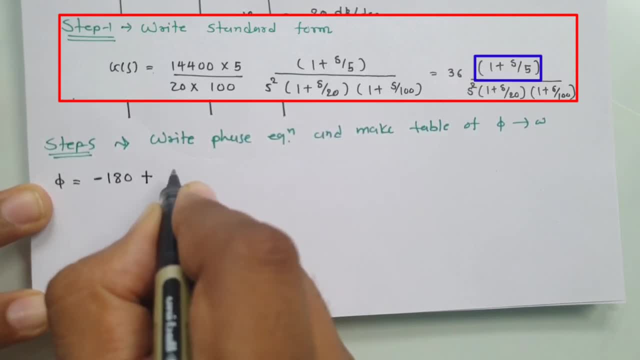 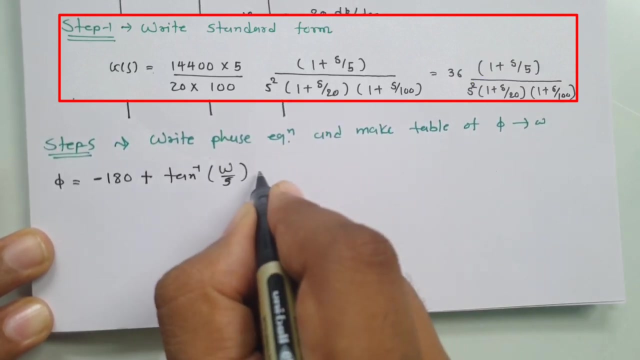 radian per second. so slope is plus and phase is also plus and phase will be plus 10 inverse omega by 5. after that, you see, there is pole at 20, so for that phase will be minus 10 inverse omega by 20, so for that phase will be minus 10 inverse omega by 20. 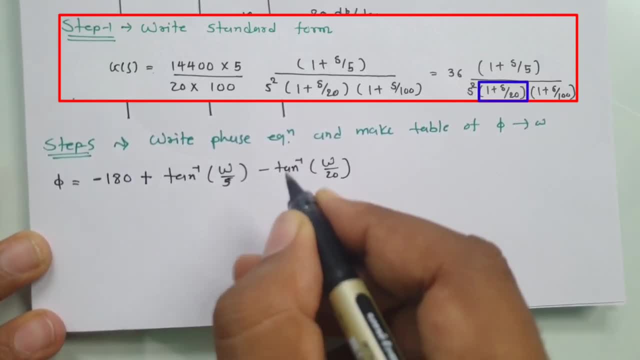 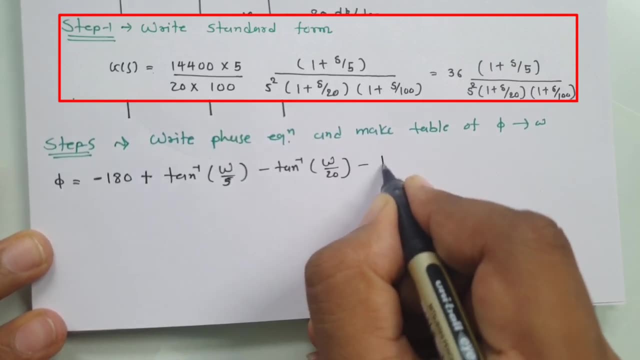 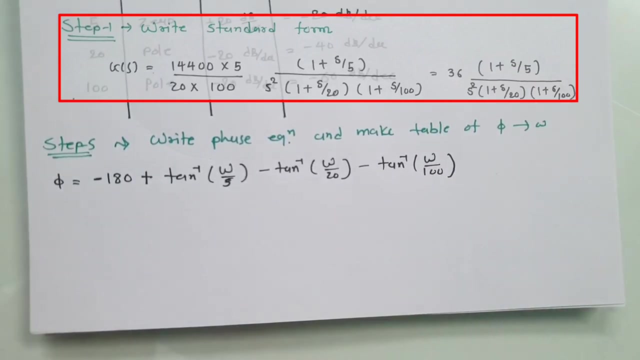 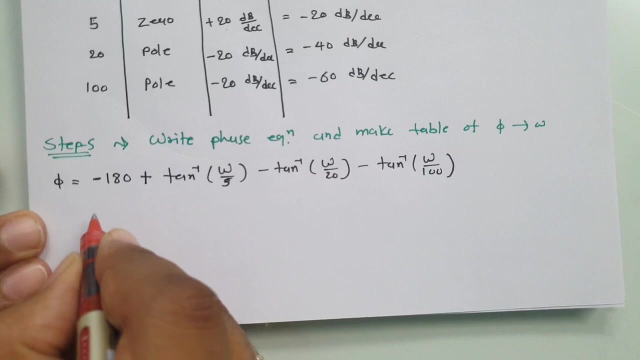 phase is negative for pole and if you see there is pole at 100, so phase will be minus for pole. 10 inverse omega by 100. so this is our phase equation. now here i'll show you how to make a table of phase. so omega that we will be changing with respect to phase we will 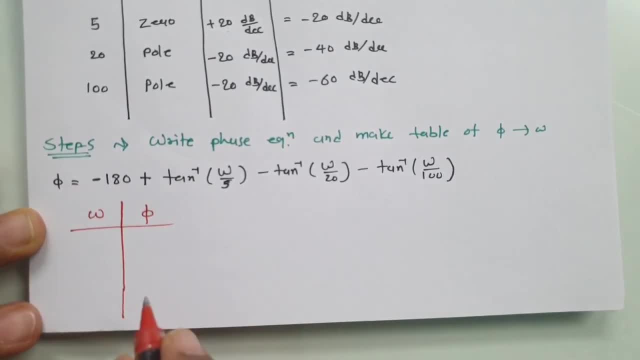 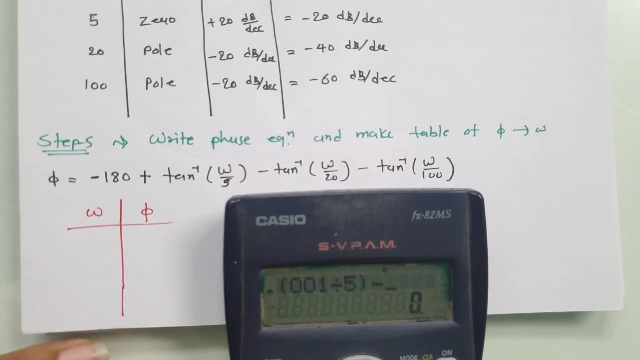 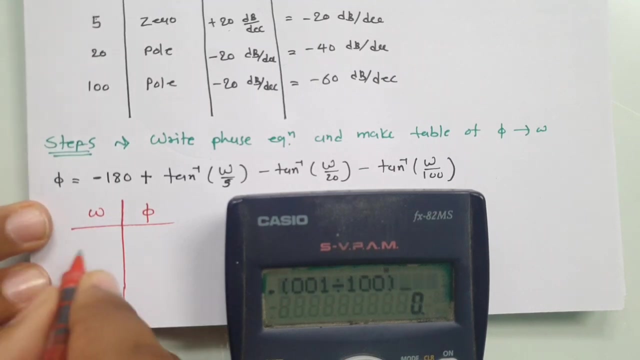 calculate, right. so let us calculate phase now. first i'll calculate phase, for omega is equals to one radian per second, and i have written the formula. so let me calculate that that is minus 172. right now, all i need to do is i just need to say it is minus 172. so next time i'll place: omega is equals to phi. now you see in. 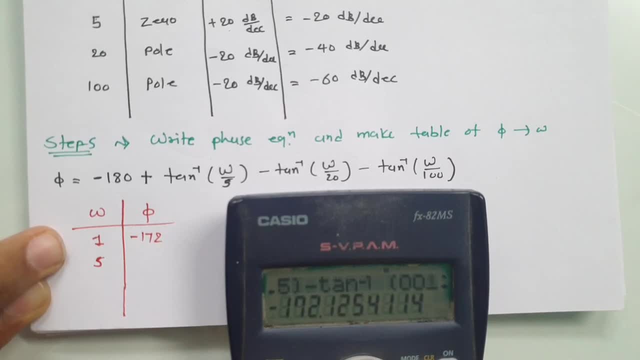 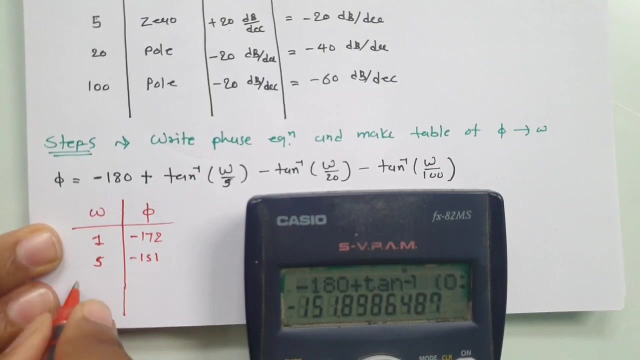 this equation, only i'm just going to change that. so now i'm just changing one with phi, and now at phi phase is minus one phi one. right now, again, i'm going to have few more values, so omega is equals to 10. that i'm considering. so 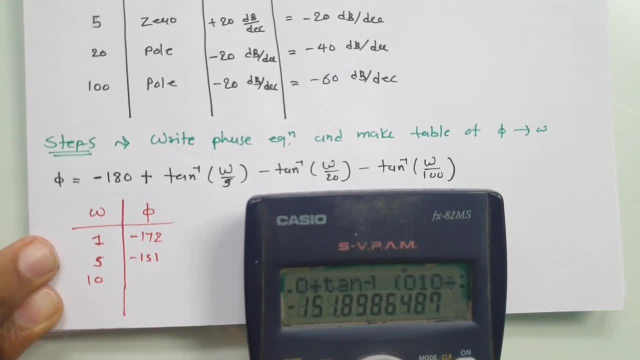 now i just need to place 10 instead of omega, you see. so every time i'm not writing this equation in calculator, i'm just changing the value in calci and i'm having values. you see now, next is minus 148. now let me place: omega is equals to phi, and i'm just changing the value in calci. 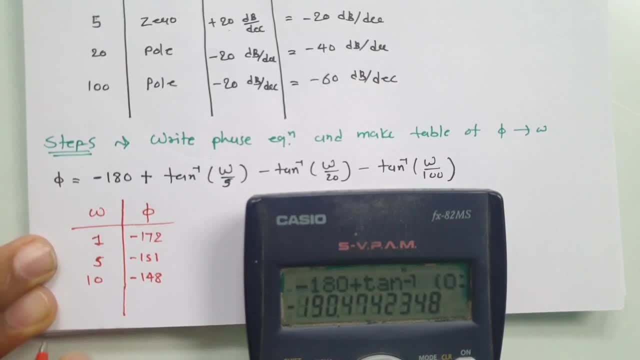 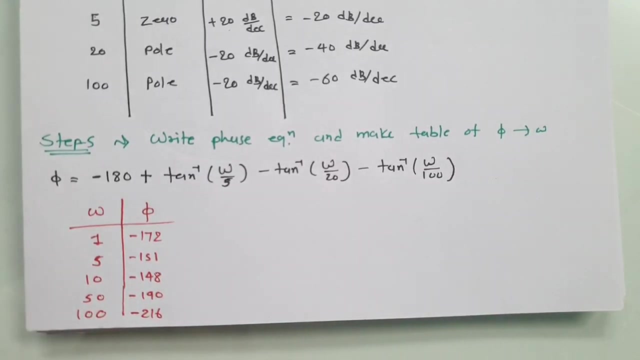 phase 50. so that is having minus 190. now let me place one more value, that is 100 and 400. frequency phase is minus 216. see here. this is not compulsory to have 5 point or 6 point or 10 point, it is based on the plot. 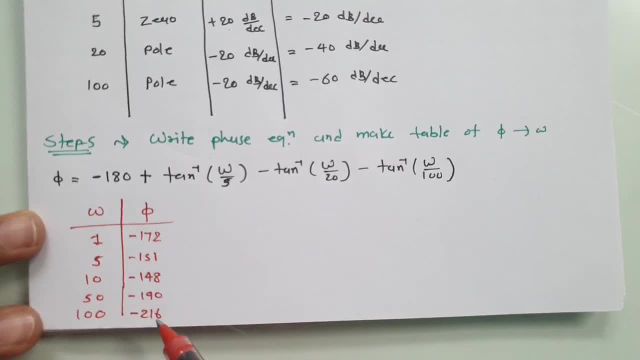 so if i don't have proper precision in plotting, then i'll be taking more points right, so it is not compulsory. what are the points that i need to take? i am- i am just choosing this randomly, so i have followed all five steps. now i need to draw body plot right, so let me take 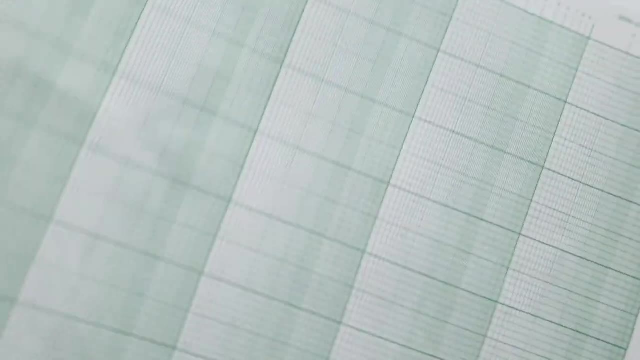 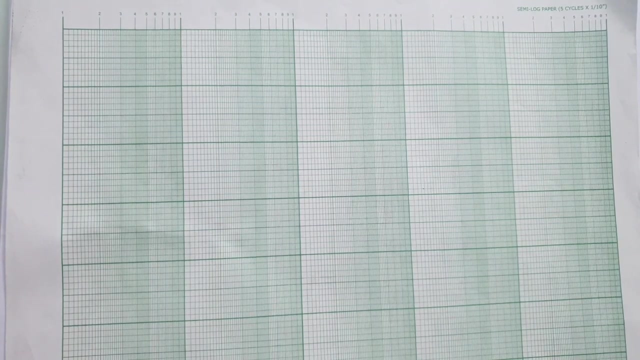 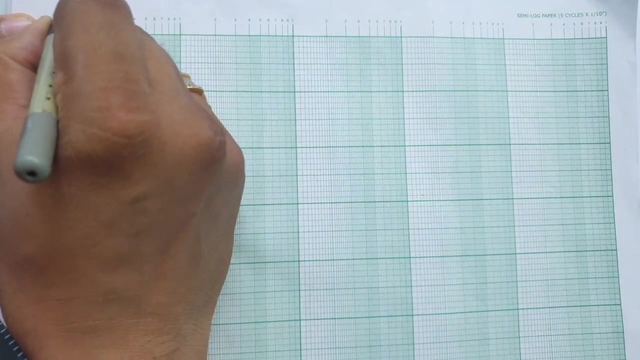 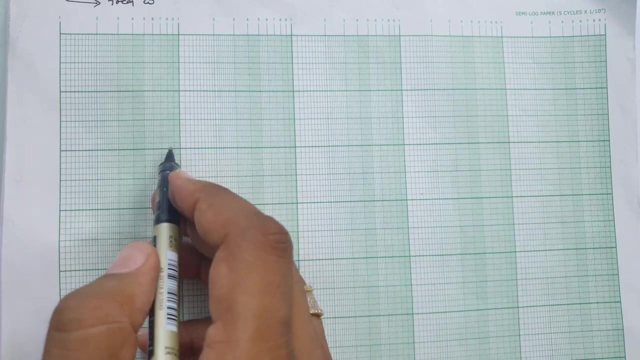 semi-lock graph paper and i'm just going to plot body plot step by step now in semi-lock graph paper. first of all, we should know: see, on horizontal axis we'll be taking frequency, and here you need to understand how frequencies are given. so frequencies are given. 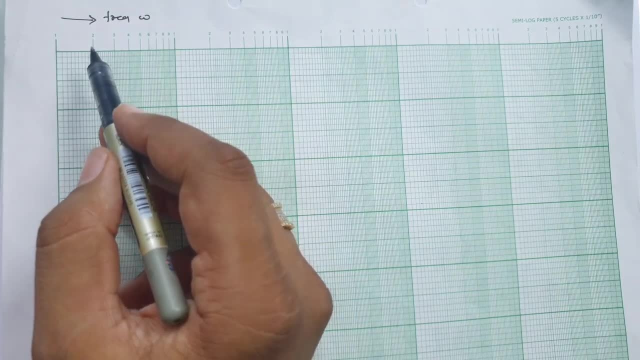 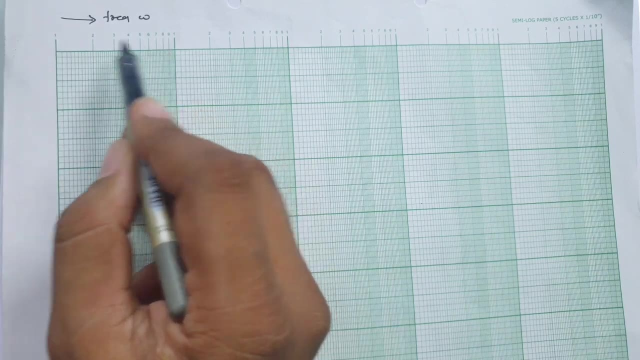 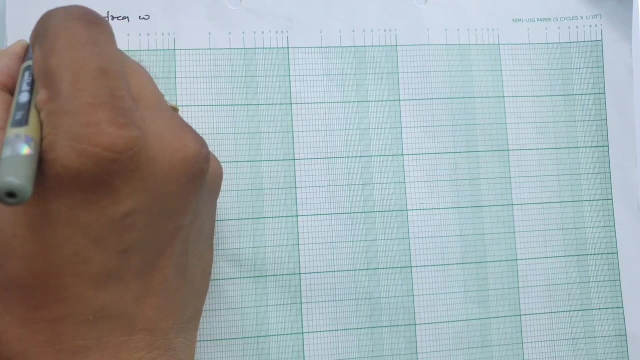 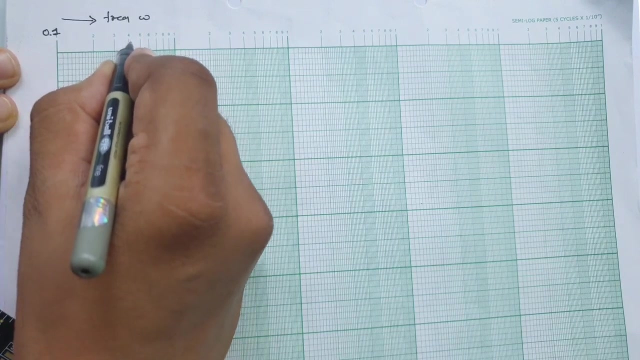 as per semi-lock value. so here you can observe, semi-lock is having one decade like this where if i consider a value of frequency to be 0.1 over here, then see here it will be 0.2, 0.3, 0.4, 0.5. 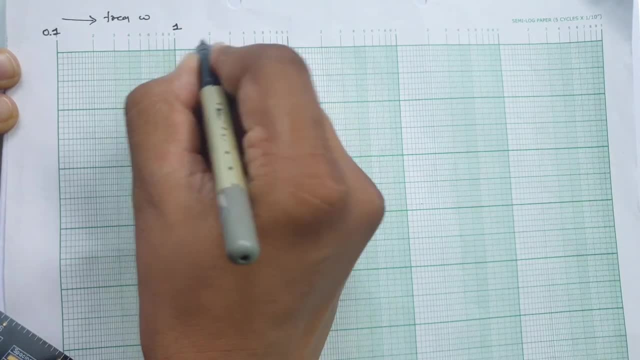 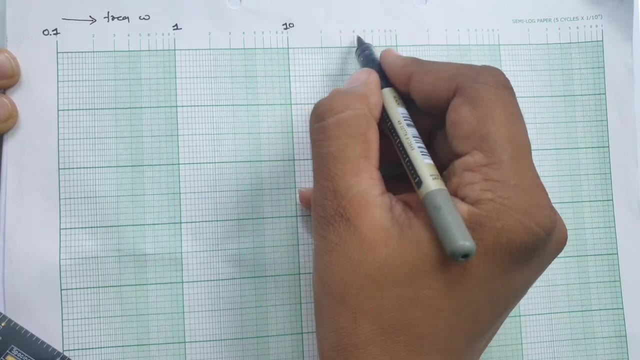 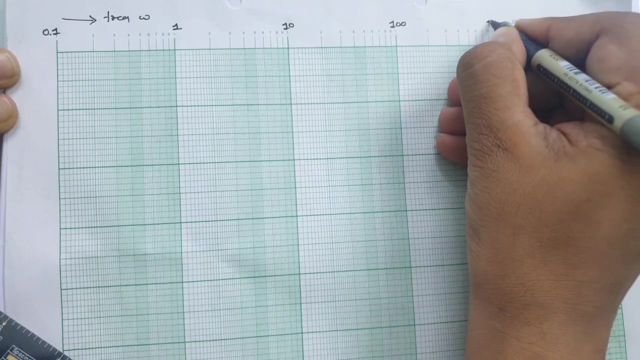 up to here it will be 1, then 2, 3, 4, 5. up to here it will be 10, then 20, 30, 40, 50. up to here it will be 100, then 100, 200, 300, 400. here it will be 1000. 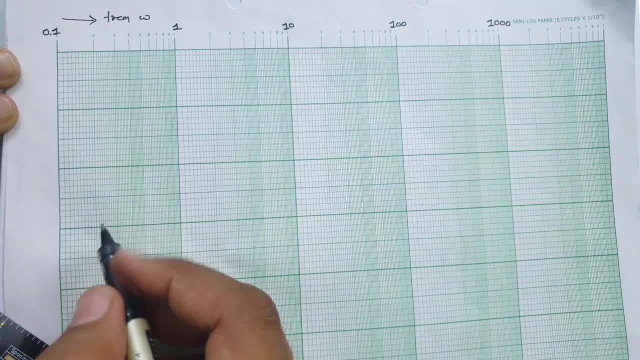 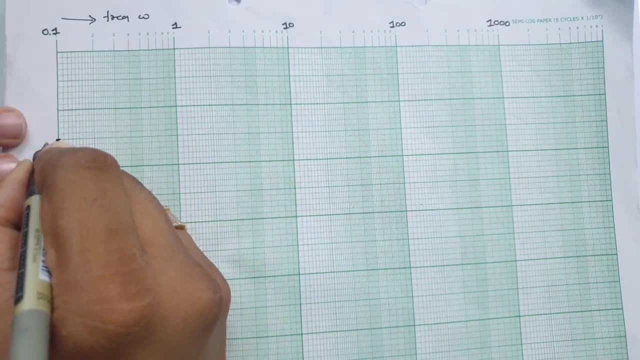 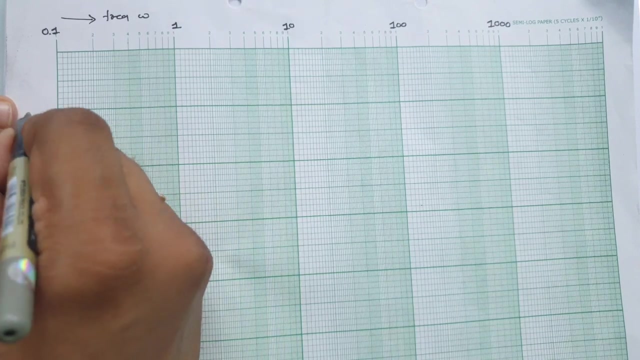 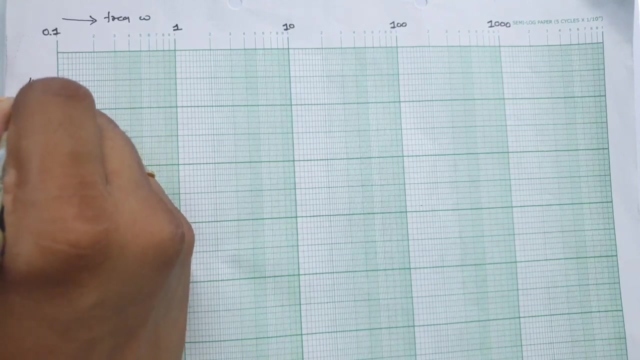 see, this is how semi-lock graph paper is there. now. first we'll be plotting gain plot. so here let us see, this is our 0 db reference, right? so here i'm just considering this as a 20, this as a 40 db and this as a 60 db. you see the scale properly. 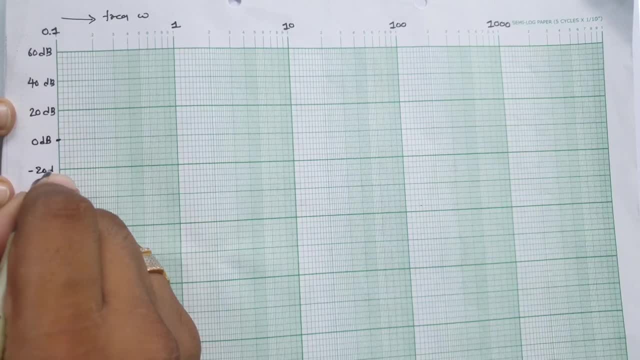 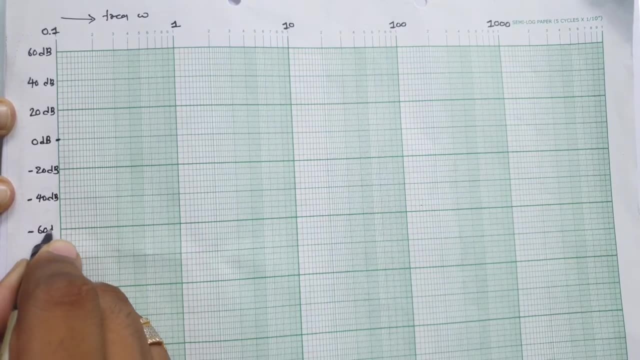 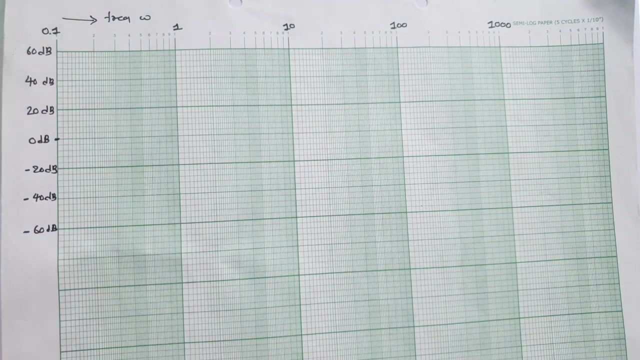 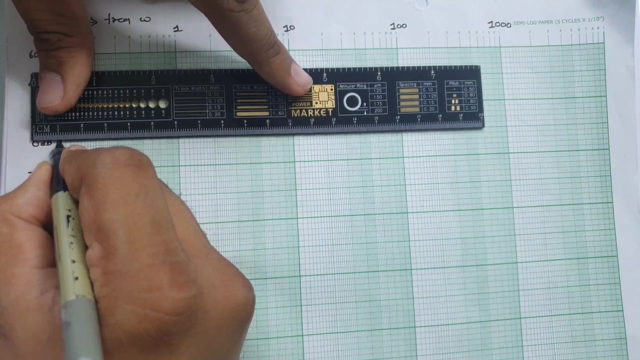 and here my scale is minus 20 db, minus 40 db, minus 60 db. that is how i have considered. right now, all i am doing is i am just stretching 0 db line. as at 0 db line, there will be gain cross. 0 db line: as at 0 db line, there will be gain cross. 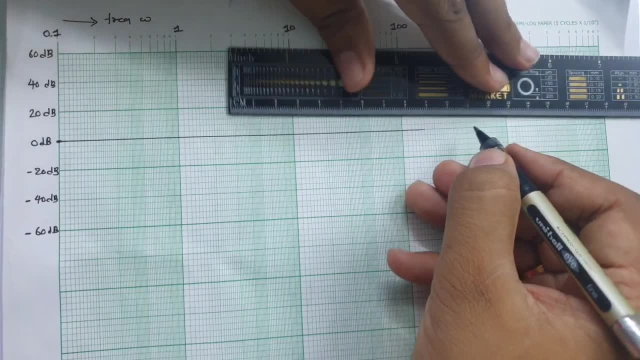 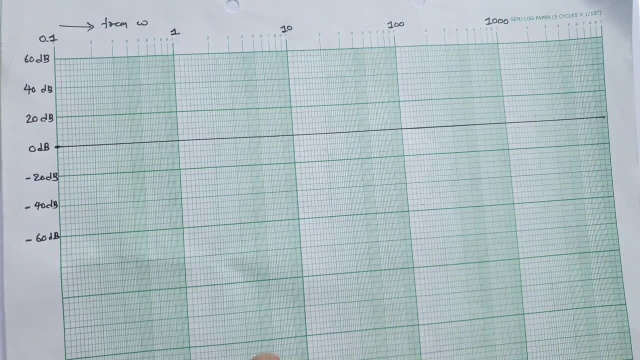 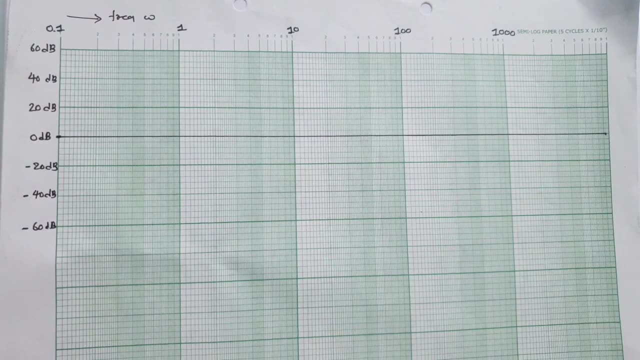 so i need to stretch 0 db line. as you can see, now we have solved all the steps. so, one by now, we have solved all the steps. so one by now, we have solved all the steps. so one by one, one one. i'll place it over here. 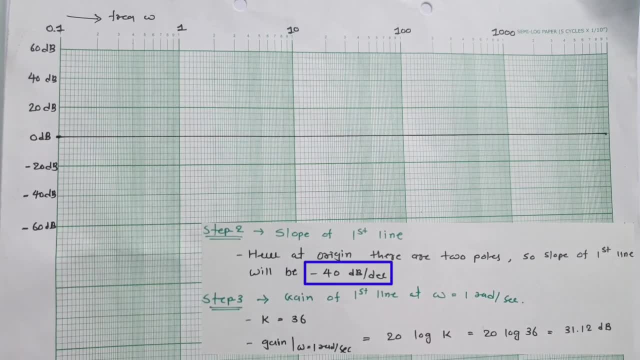 i'll place it over here. i'll place it over here. so first line slope is minus 40 db per so. first line slope is minus 40 db per so. first line slope is minus 40 db per decade. first line slope is decade. first line slope is: 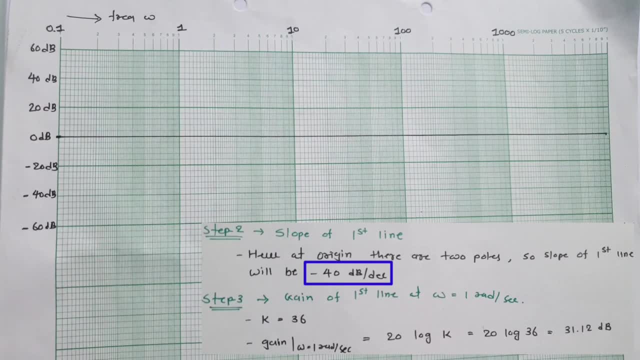 decade, first line slope is minus 40 db per decade, minus 40 db per decade, minus 40 db per decade. and if you observe, and if you observe, and if you observe gain at one radian per second, gain at one radian per second, gain at one radian per second, then gain at one radian per second. 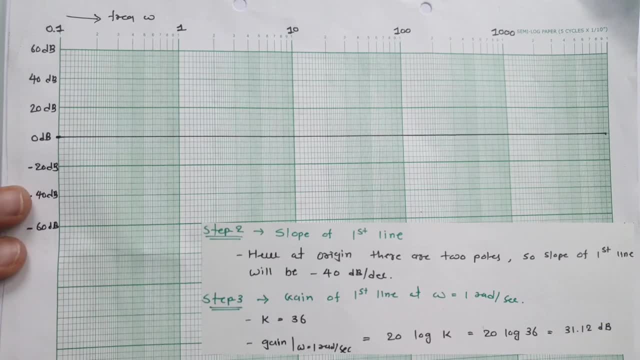 then gain at one radian per second, then gain at one radian per second was 31.12, was 31.12, was 31.12, right, so you see, right, so you see right, so you see, this is one radian per second, this is one radian per second. 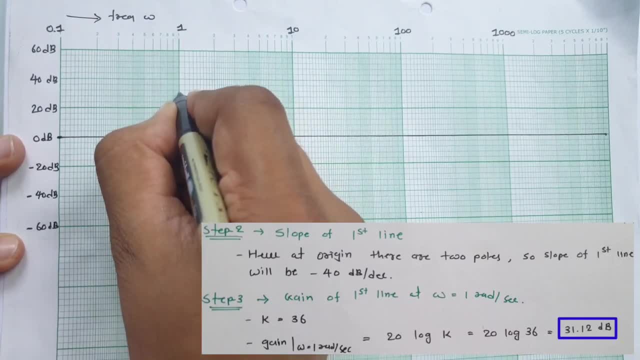 this is one radian per second, and 31.12 that is happening, and 31.12 that is happening, and 31.12 that is happening somewhere over here, somewhere over here, somewhere over here, right, right, right. so this is what the point. so this is what the point. 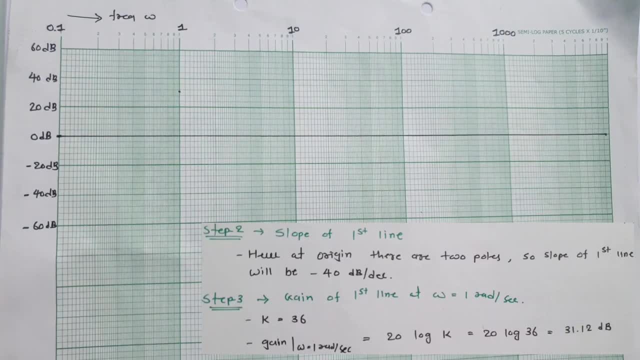 so this is what the point, and that point should have, and that point should have, and that point should have: minus 40 db per decade. minus 40 db per decade, minus 40 db per decade. slope now to plot first line. slope now to plot first line. 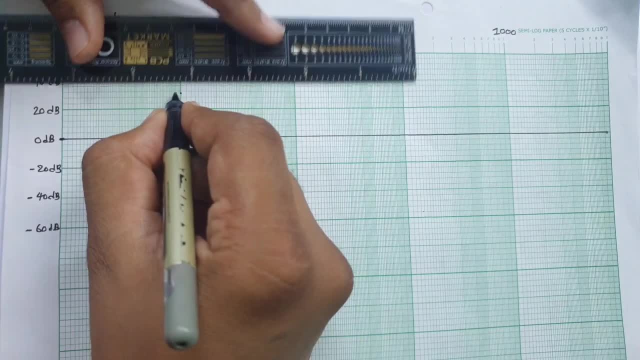 slope. now to plot first line. you see, this is one. you see this is one. you see this is one decade, right here to here. decade, right here to here. decade, right here to here. there is one decade and here to here. there is one decade and here to here. 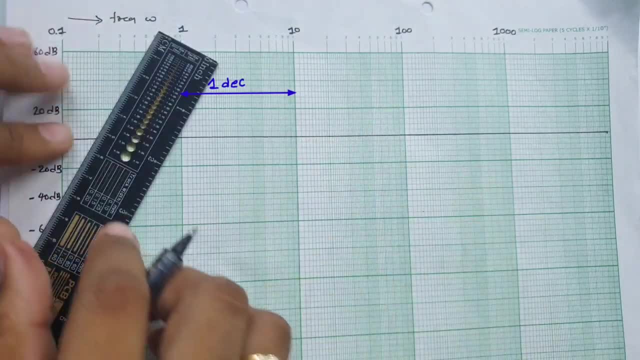 there is one decade, and here to here, there is one decade. there is one decade, there is one decade, right and here, right and here, right and here. now, you see i have took, now you see i have took, now you see i have took a scale, a scale. 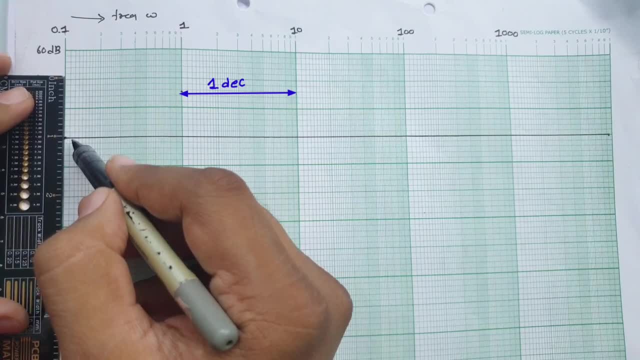 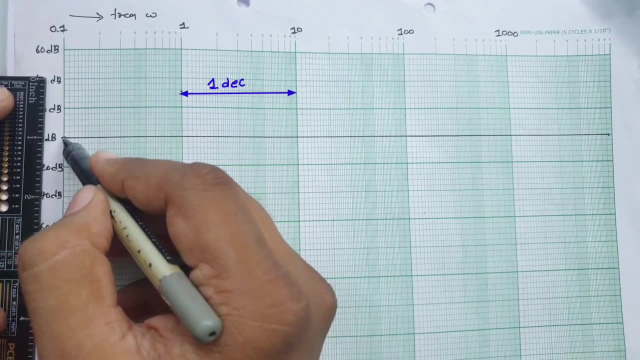 a scale where you see, where you see, where you see one inch that is equals to 40 db. you one inch that is equals to 40 db, you one inch that is equals to 40 db. you see this is inch, see this is inch, see this is inch. and here, if you observe, this is 0 db. 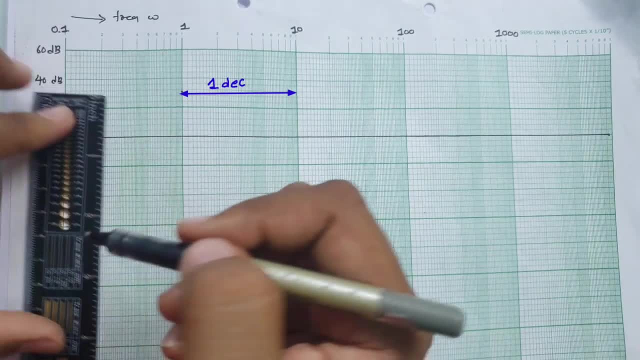 and here, if you observe, this is 0 db. and here, if you observe, this is 0 db and this is 40 db. so one inch is equals and this is 40 db. so one inch is equals and this is 40 db. so one inch is equals to 40 db. 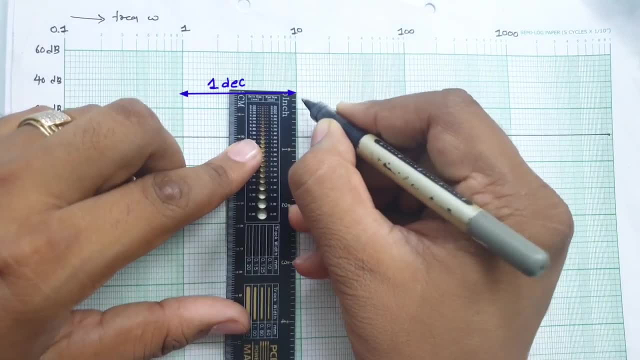 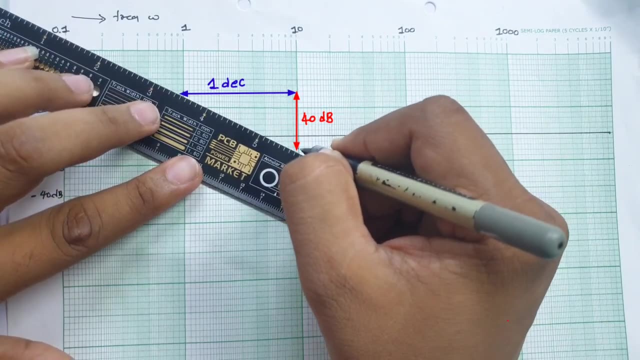 to 40 db to 40 db, right, so here to one inch, right. so here to one inch, right, so here to one inch. i need to take like this, i need to take like this, i need to take like this, right, and i'm just stretching a line. 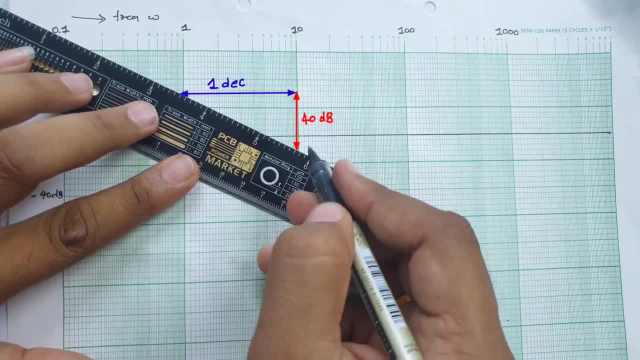 right, and i'm just stretching a line right, and i'm just stretching a line from one decade. you see, from one decade. you see, from one decade. you see, here to here, there is one decade, so i'm here to here, there is one decade, so i'm. 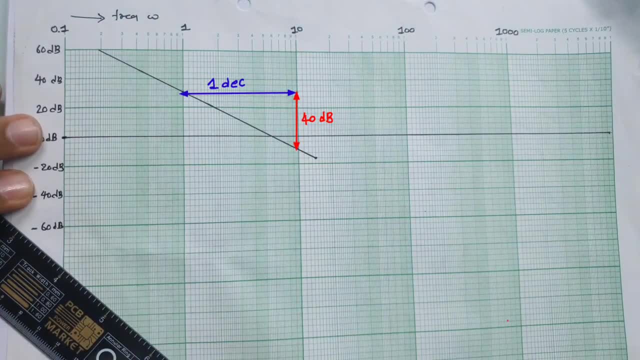 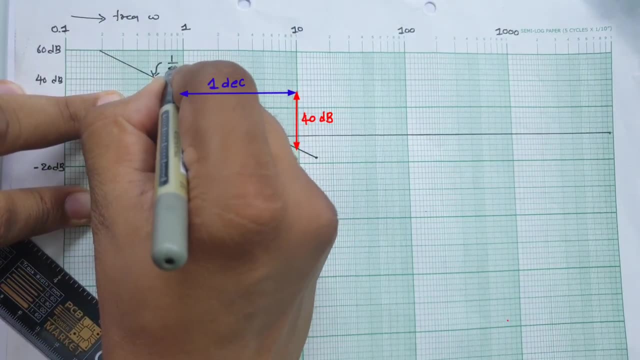 here to here, there is one decade. so i'm just stretching a line, just stretching a line. so i'm just stretching a line, just stretching a line, first line, and that is a line which is first line, and that is a line which is first line, and that is a line which is 1 by s square line. 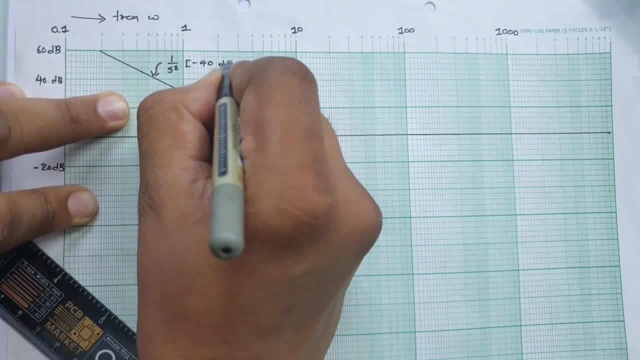 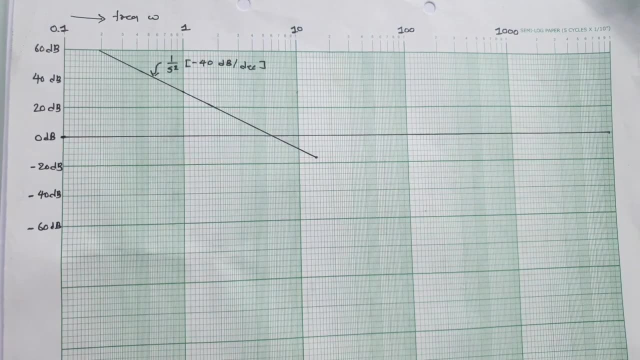 1 by s square line. 1 by s square line that is having slope minus 40. that is having slope minus 40. that is having slope minus 40. db per decade. db per decade, db per decade. right now, right now, right now. we need to see next. 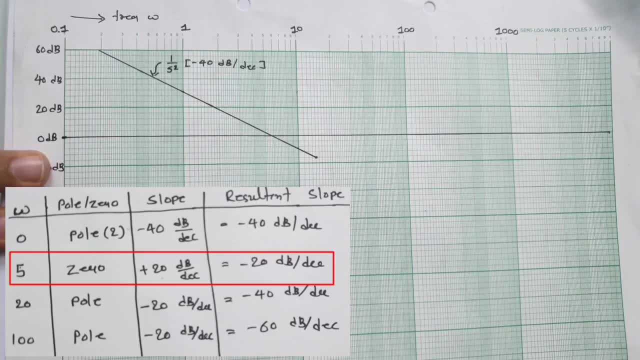 we need to see next. we need to see next corner frequency, corner frequency, corner frequency and next corner frequency that is, and next corner frequency that is, and next corner frequency that is happening, happening, happening at five radian per second, so you see, at five radian per second, so you see. 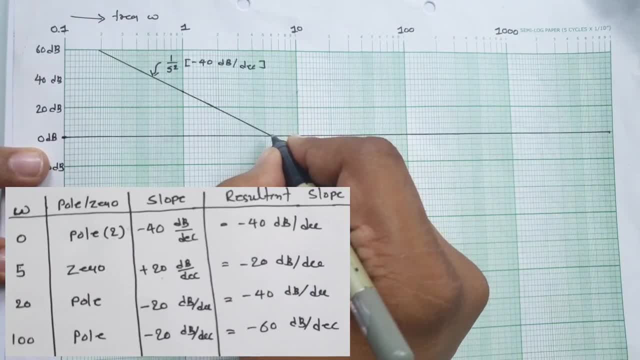 at five radian per second. so you see, five radian per second, that is happening. five radian per second, that is happening. five radian per second, that is happening somewhere over here, somewhere over here, somewhere over here. 5 radian per second, 5 radian per second. 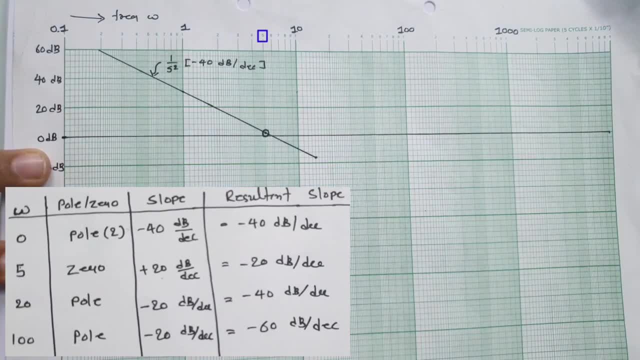 5 radian per second. so make a bubble over there. so make a bubble over there. so make a bubble over there. so this is 5 radian per second. so this is 5 radian per second. so this is 5 radian per second, and at 5 radian per second you can. 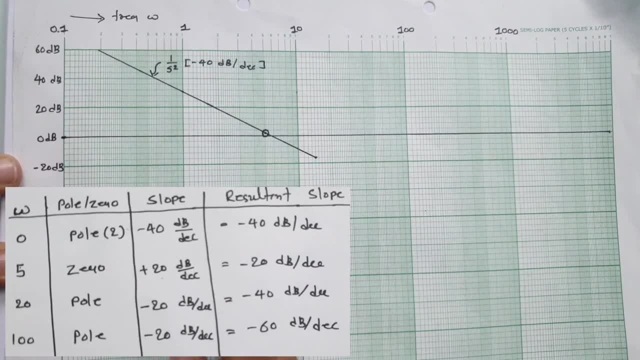 and at 5 radian per second you can, and at 5 radian per second you can observe, observe, observe. resultant slope is resultant slope is resultant slope is minus 20 db per decade, minus 20 db per decade, minus 20 db per decade, so plus 5. 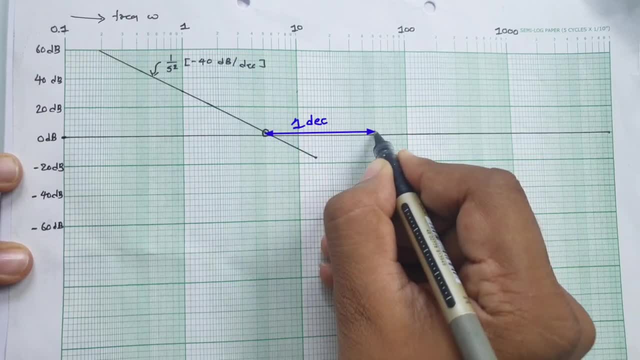 so plus 5, so plus 5 to 5. we need to to 5, we need to to 5, we need to stretch horizontally like this stretch horizontally, like this stretch horizontally, like this. and from here we need to see, and from here we need to see. 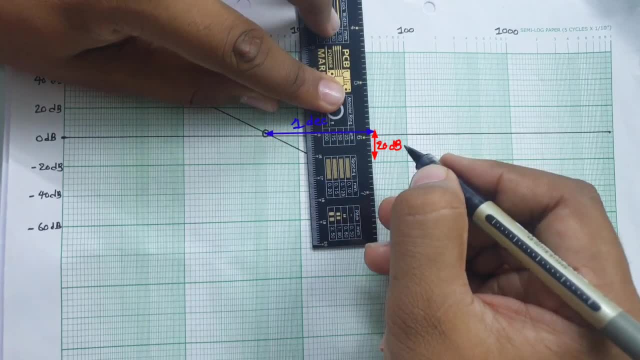 and from here we need to see that minus 20 db per decade. so half of that, minus 20 db per decade. so half of that minus 20 db per decade. so half of the inch that we need to stretch, so you, the inch that we need to stretch, so you. 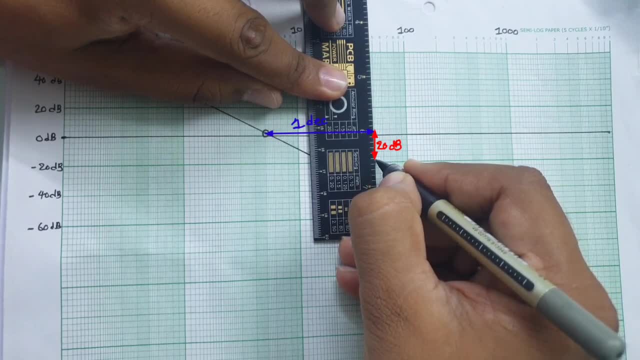 the inch that we need to stretch. so you see, see, see, here to here, there is half inch. here to here, there is half inch. here to here, there is half inch. right, right, right. so i'm taking a point over here. so i'm taking a point over here. 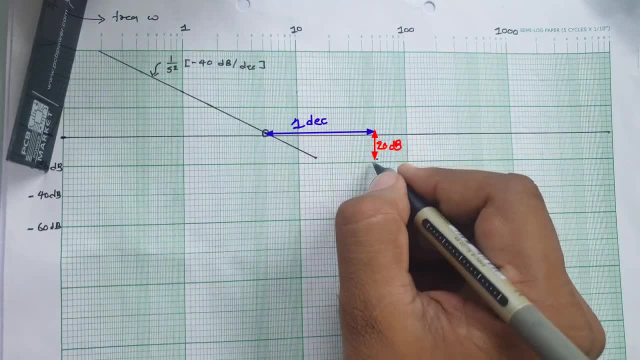 so i'm taking a point over here. so 5 to 5, so 5 to 5, so 5 to 5 and half inch means 20 and half inch means 20 and half inch means 20 db down. so minus 20 db per decade. 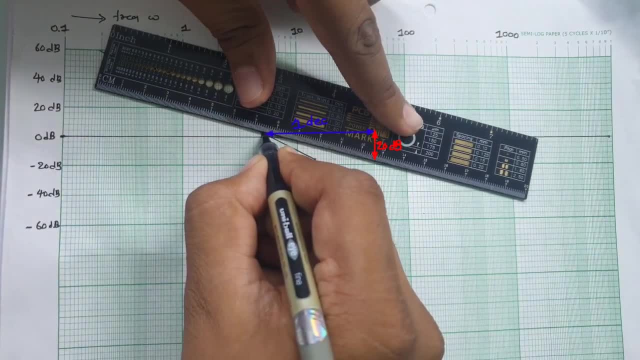 db down, so minus 20 db per decade. db down, so minus 20 db per decade. slope: that will happen. so from this point, slope: that will happen. so from this point, slope: that will happen. so from this point to this point, i am stretching a line. to this point, i am stretching a line. 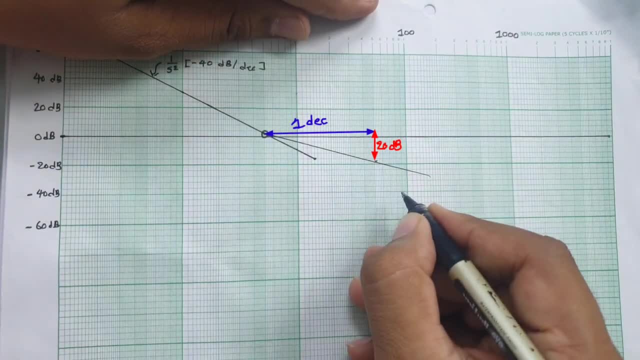 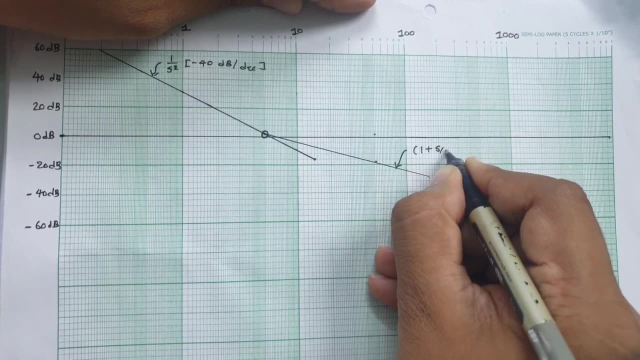 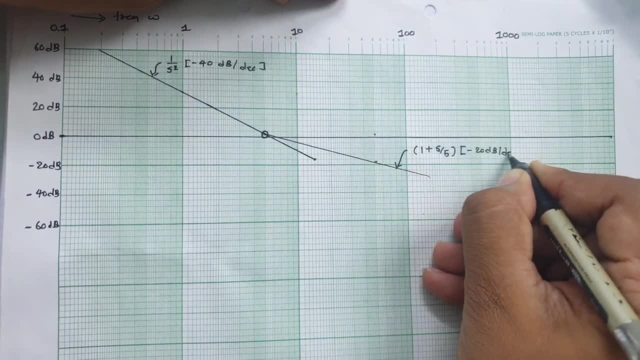 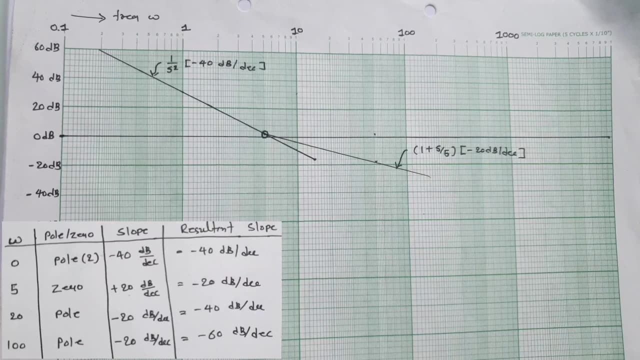 that is having a slope, that is having a slope minus 20, minus 20, minus 20 db per db, per db per decade, decade, decade, right, right, right now. next line, now, next line, now, next line. that is that is there, with corner frequency 20. so you see, this is 10 and this is 20, so that is happening somewhere. 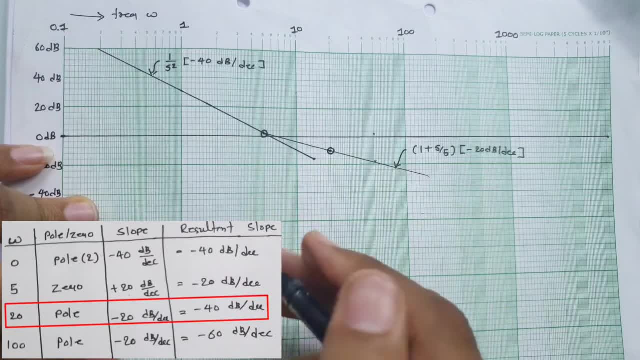 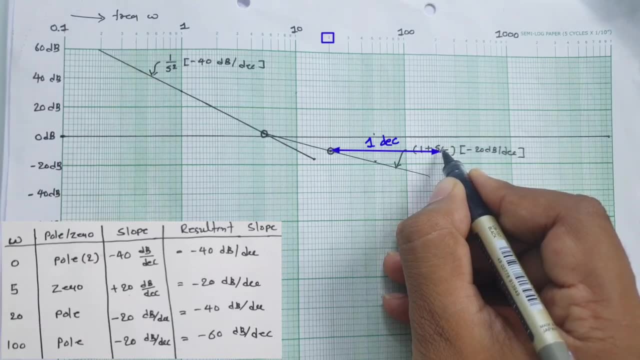 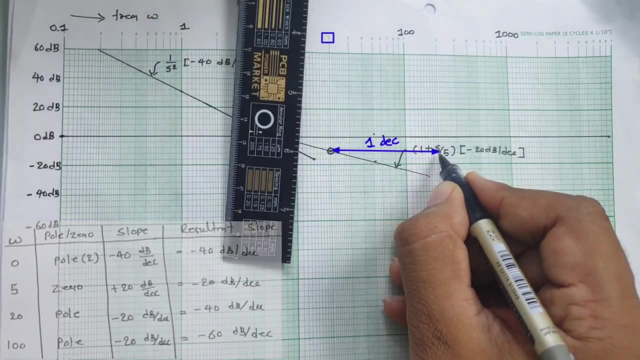 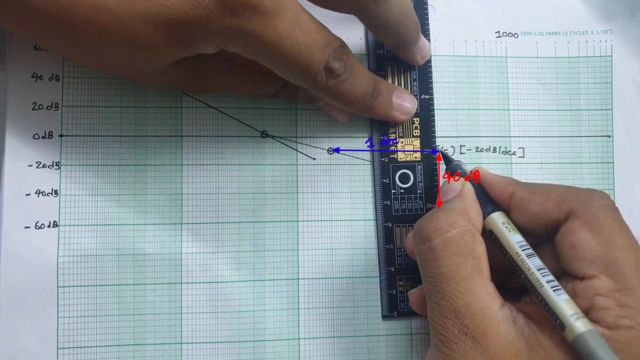 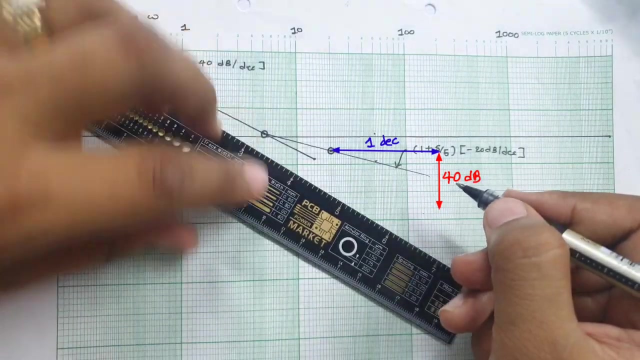 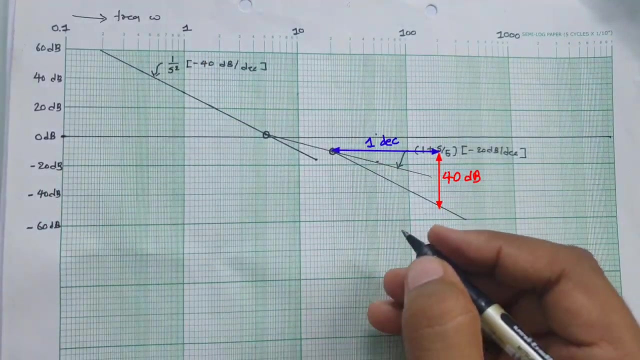 over here. so this is 20, make a corner frequency and this 20 to this 20 that is coming somewhere over here and slope is minus 40 db per decade. so minus 40 means 1 inch from here. so here to 1 inch. right and see, we need to stretch a line. so this is a line which is there with 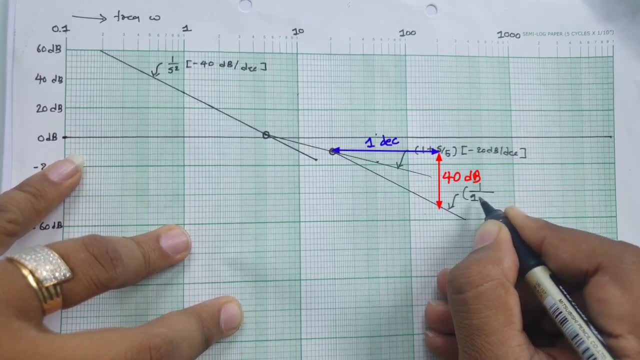 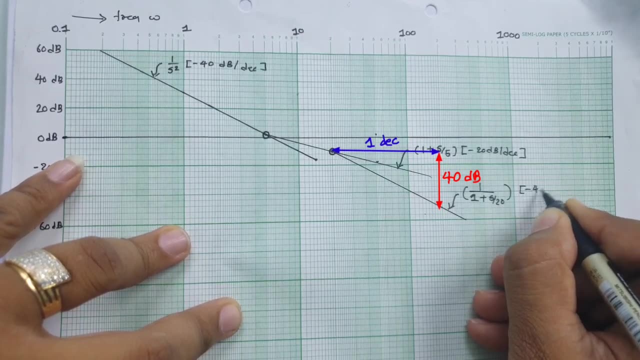 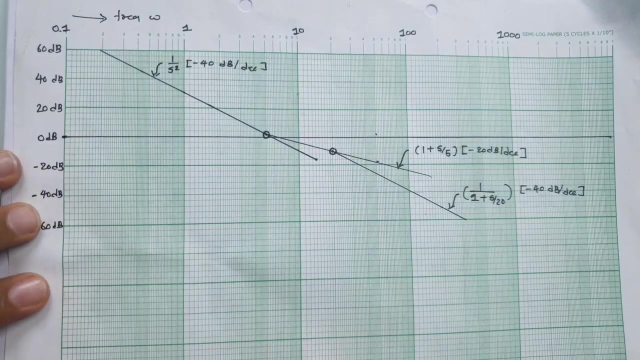 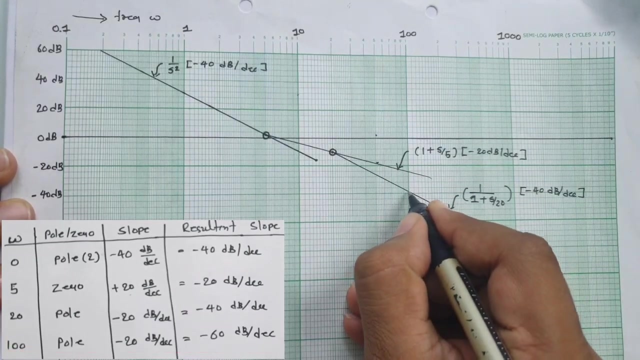 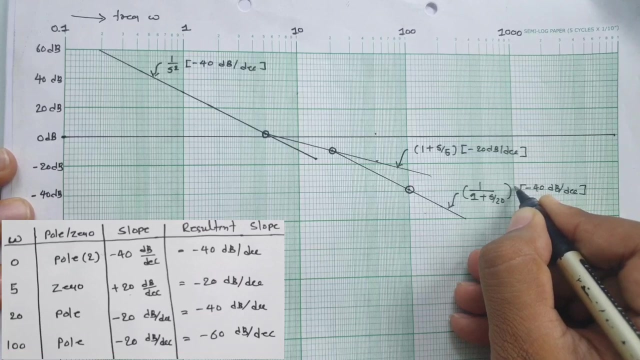 1, divide by 1 plus and s by 20, and that is having a slope minus 40 db per decade. right and last corner, frequency, that is happening at 100. so 100 is happening somewhere over here. you see. so 100 to 100. one decade is there and slope of that is: 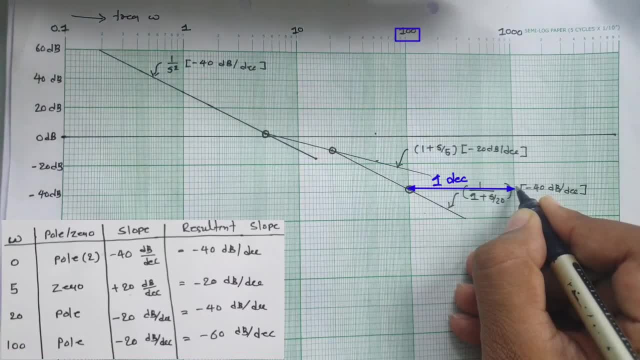 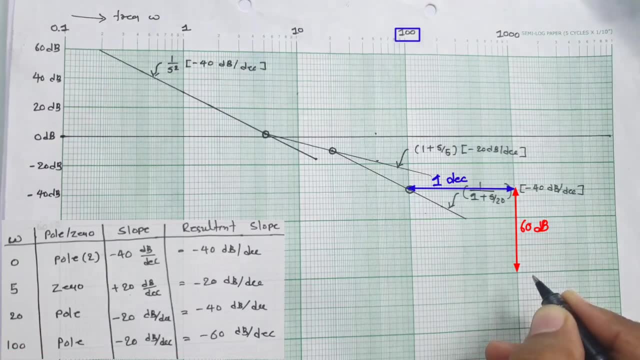 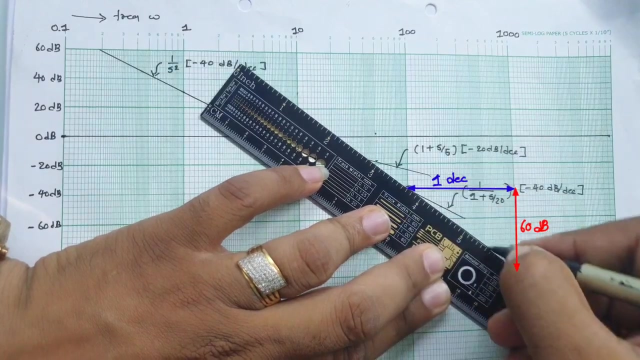 20 minus 60 db. so minus 60 means see here to here, 20, here to here, 40, here to here, that is 60. so if I stretch a line from this point, I'll be having slope which is minus 60 db per decade, right, so this. 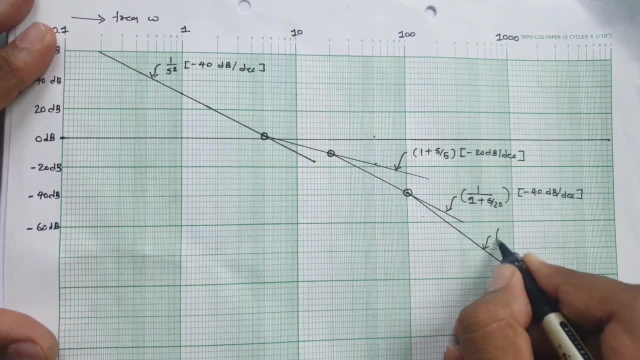 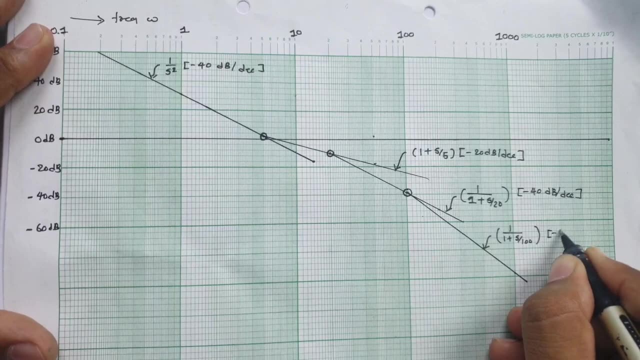 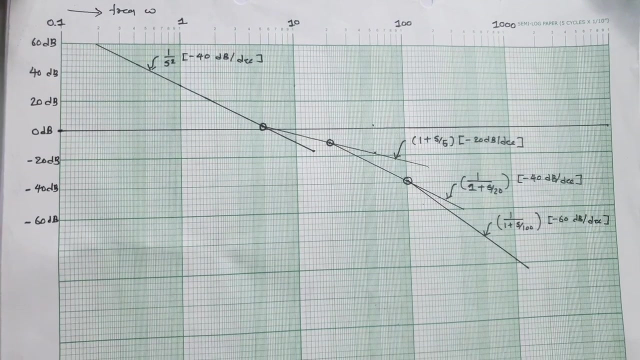 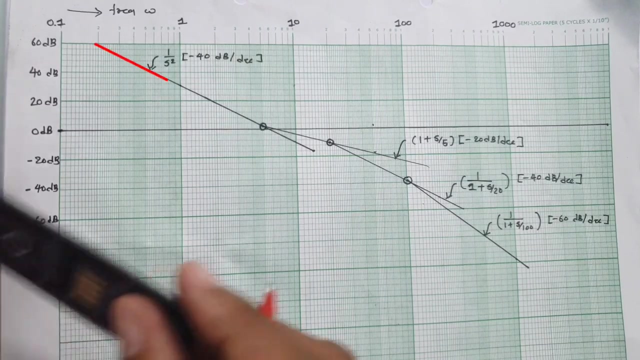 line that is a line, 1 divide by 1 plus s divide by 100, that is having a slope minus 60 dB per decade. so this is how we can have a gain plotting. now, in this gain plotting there are many extra lines that one can say right. so corner to corner. 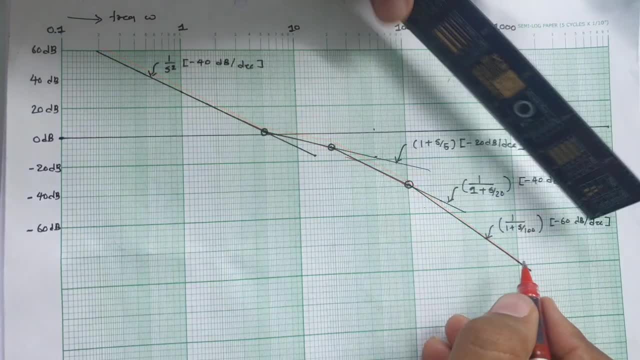 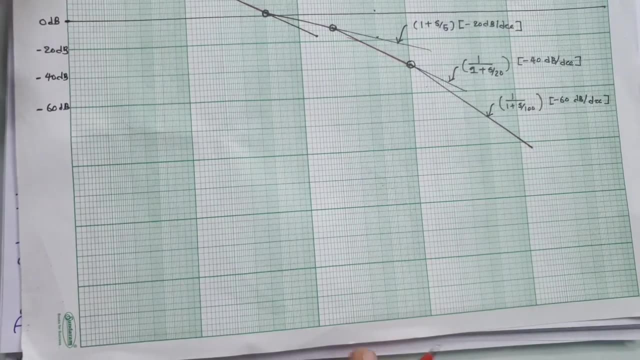 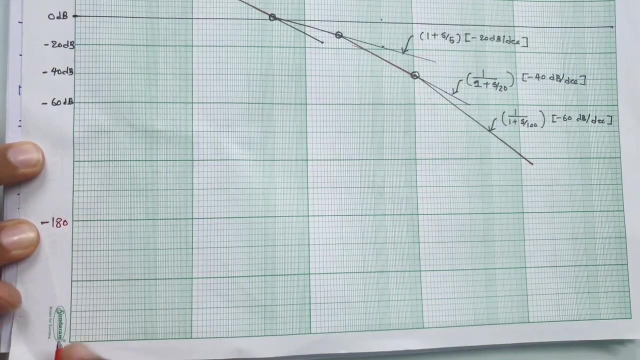 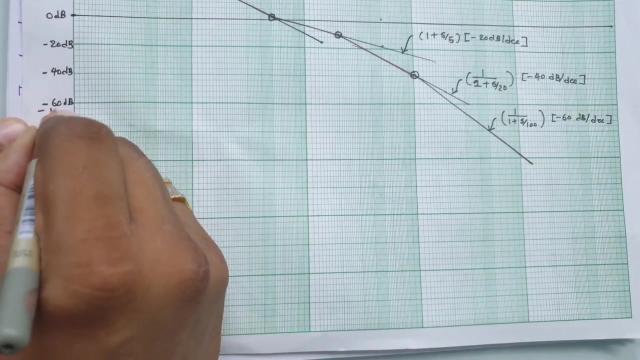 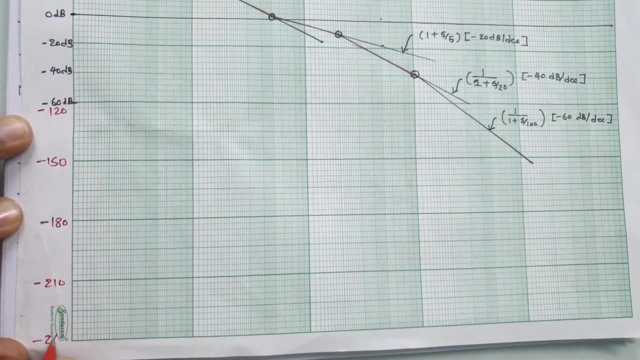 frequency graph that we need to consider. so this is actual plot of gain. right now let us have a phase plot. so for phase plot, I am considering this as a minus 180 degree, this as minus 150 degree and this as minus 120 at this point, and here minus 210, and here minus 240. that is there. 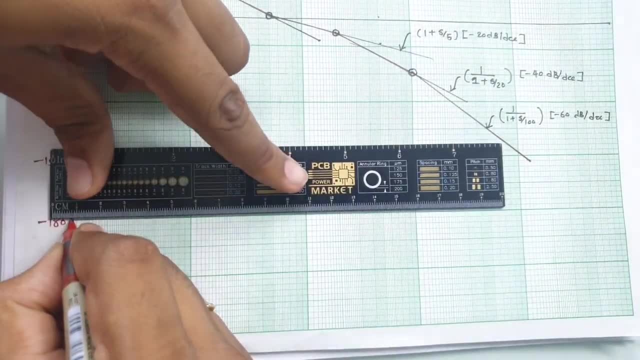 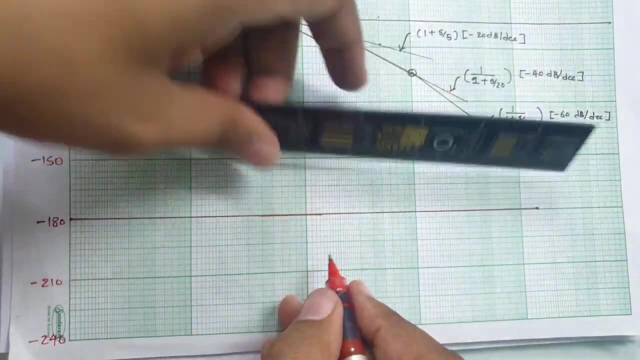 and I need to stretch a line horizontally for minus 240, and I need to stretch a line horizontally for minus 240 and I need to stretch a line horizontally for minus 180 degree, as phase crossover will happen at minus 180 degree right now. you can see the. 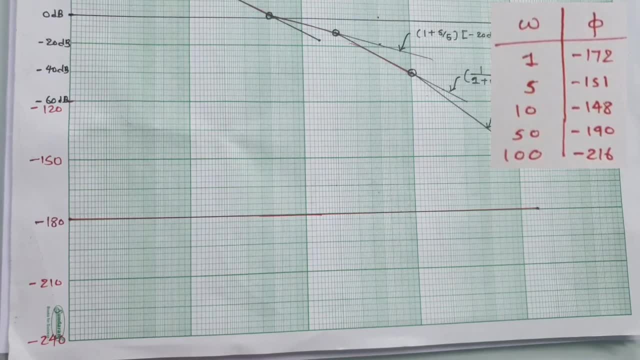 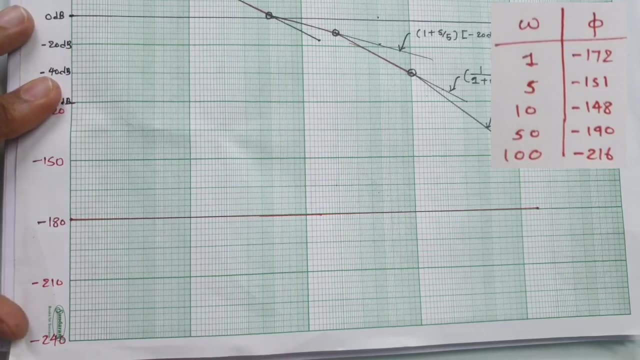 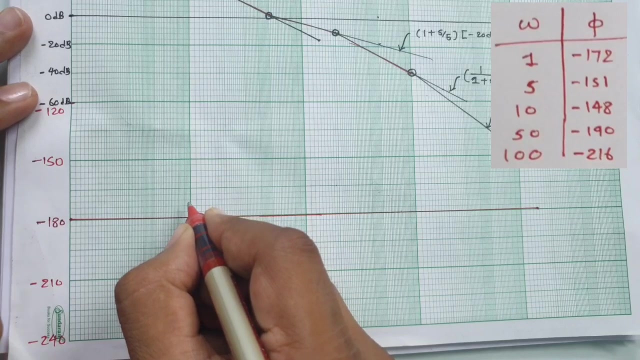 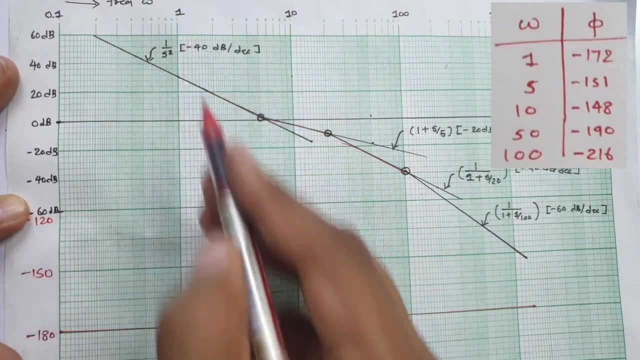 table where few values that I have noted. so at omega is equals to one, radian per second, value of phase is 172. you can see in table. so 172, that will happen somewhere over here. 172 at omega is equals to one. you see, this is: omega is equals to one and 172 that will happen. 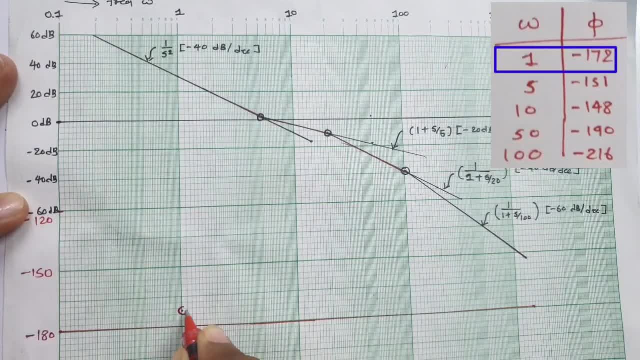 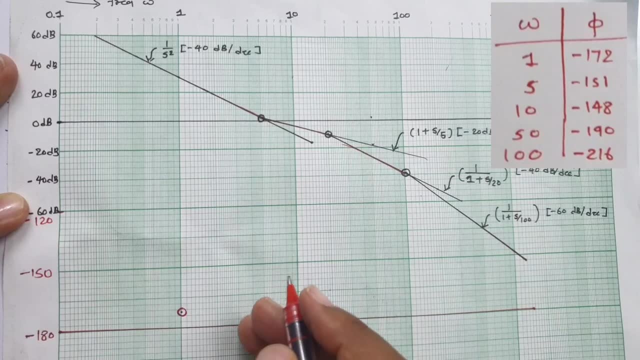 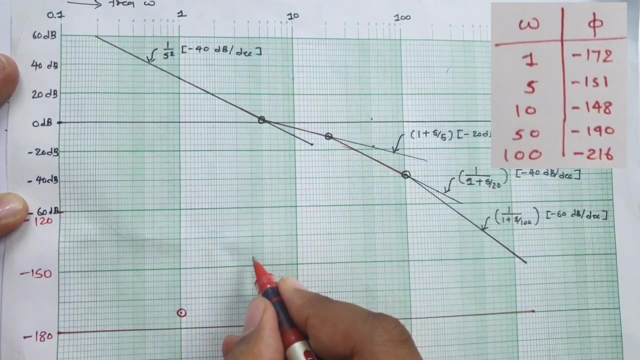 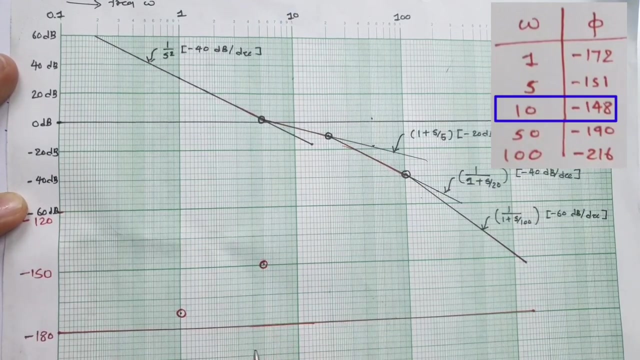 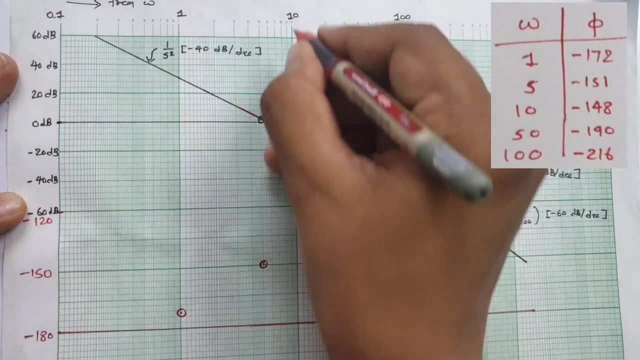 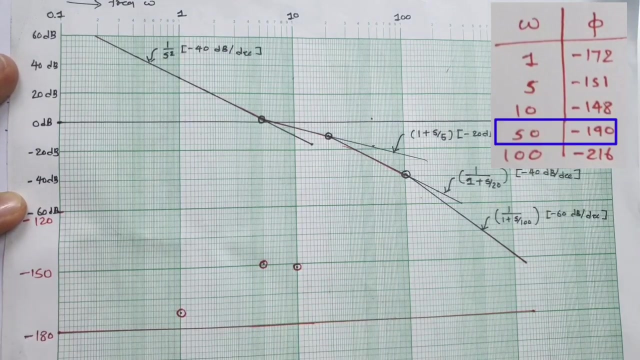 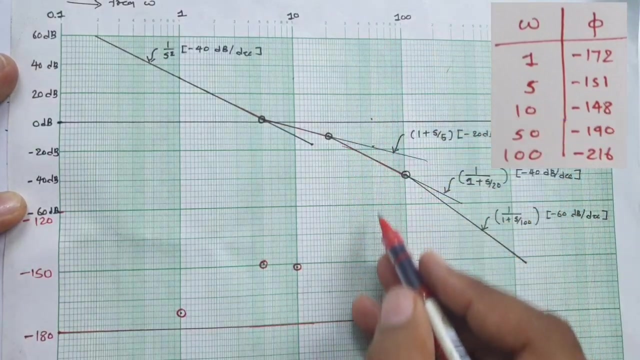 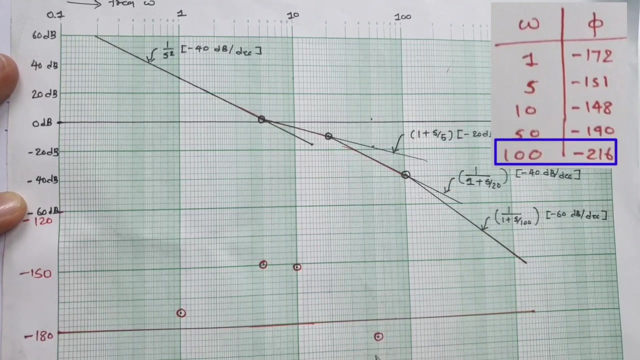 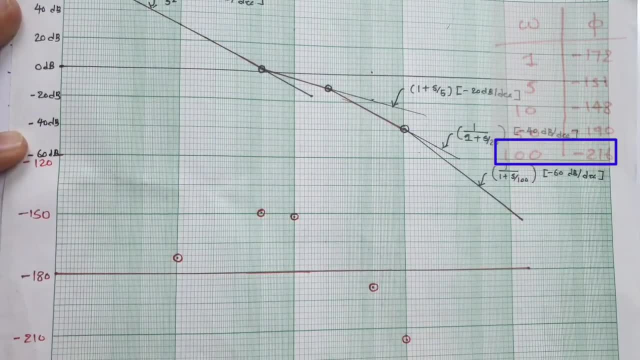 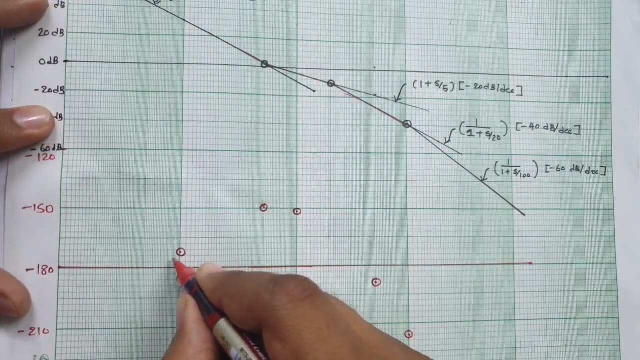 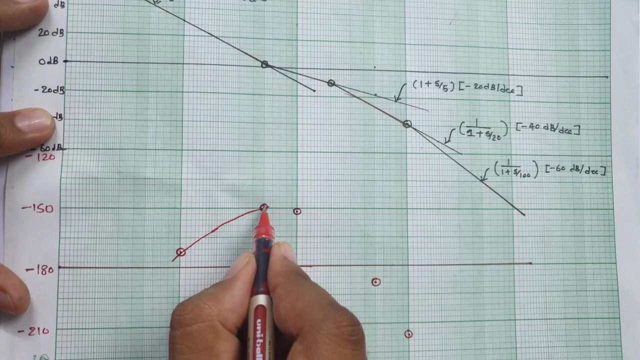 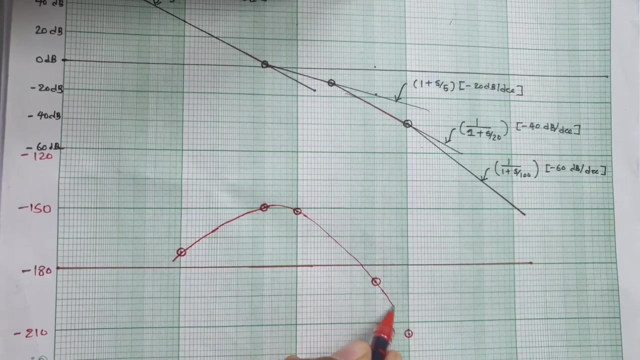 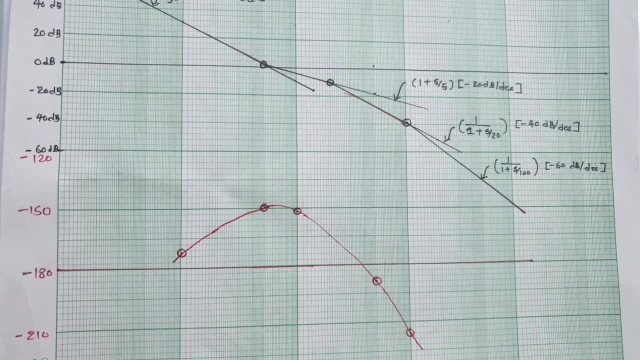 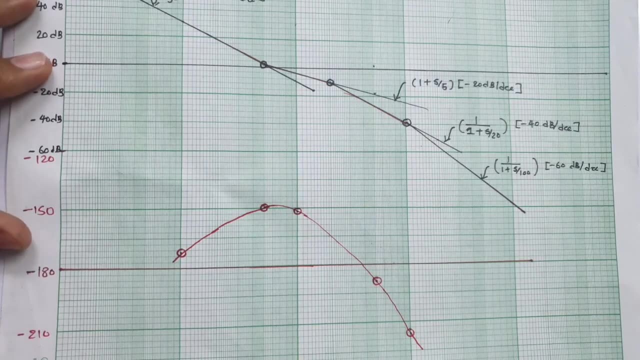 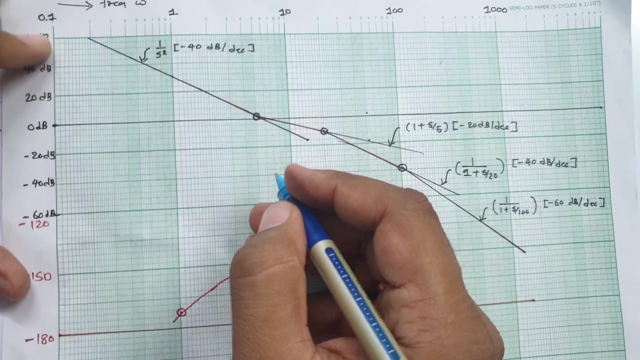 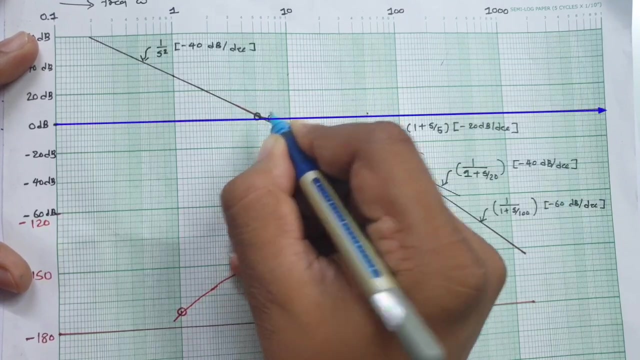 If you want to nullify human error, then you will have to take more points. right Now. all I'll be doing is I'll be identifying first what is gain crossover frequency. right, So you see, gain crossover- that is happening exactly over here. 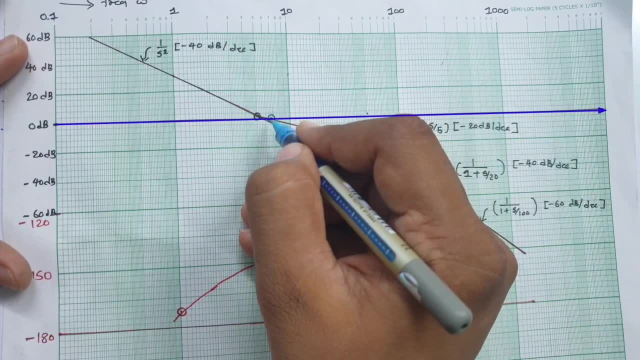 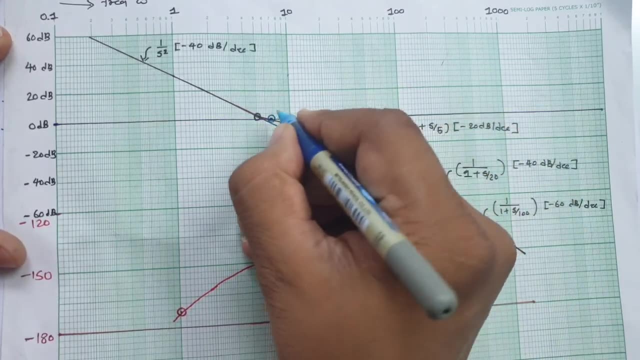 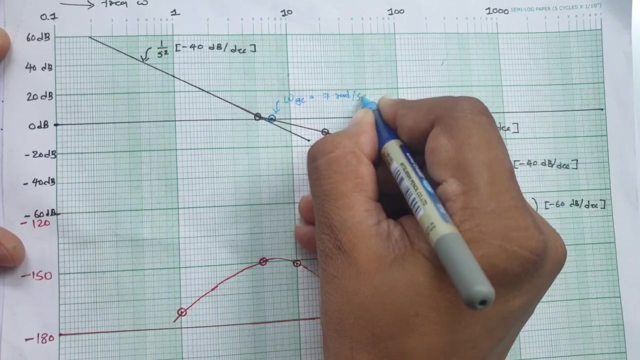 So if you see gain crossover, so that is very nearer to 7, right Gain crossover, that is very nearer to 7.. So I can say approximated value will come right. So omega gc, that is 7 radian per second. 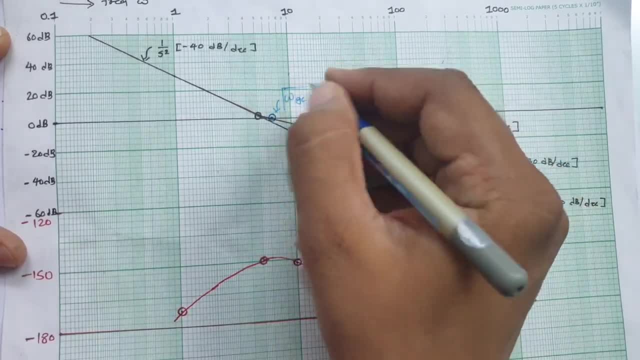 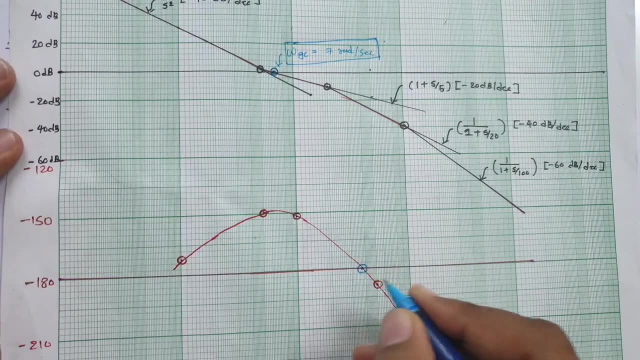 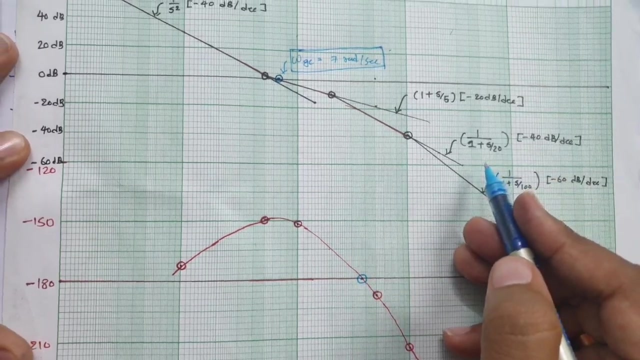 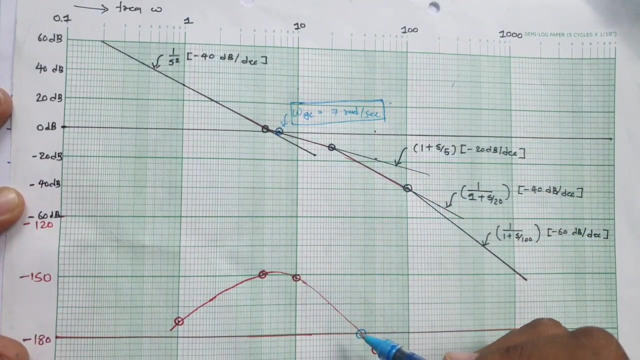 That is our first parameter of equation. Now, if you see phase crossover, so that is happening somewhere over here, right? And if you see So that is approximately 38. You see here 30 and 40 is there, So it is very near to 4 means 40, but somewhat this side, right. 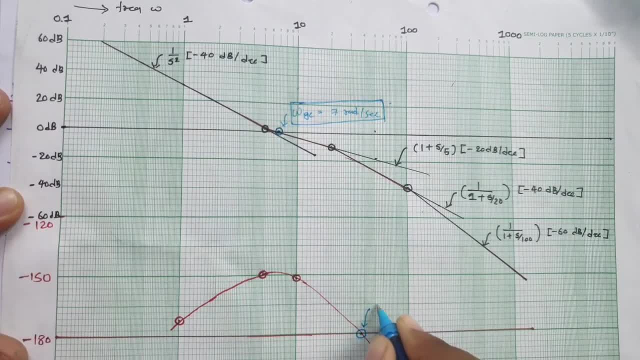 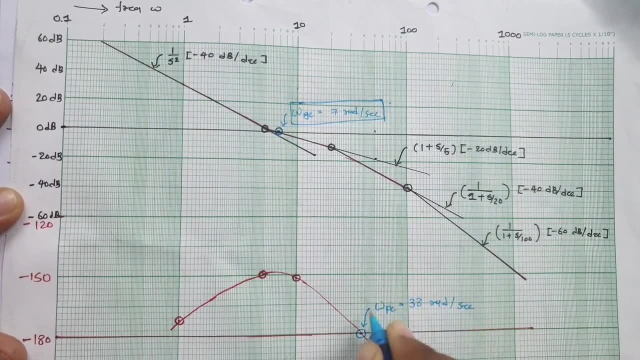 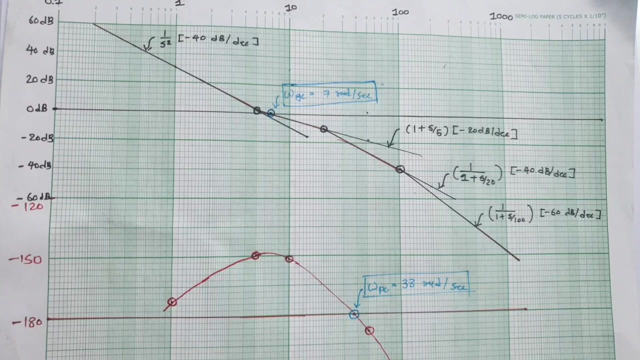 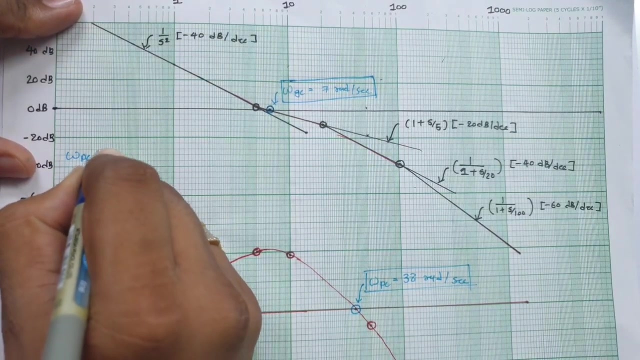 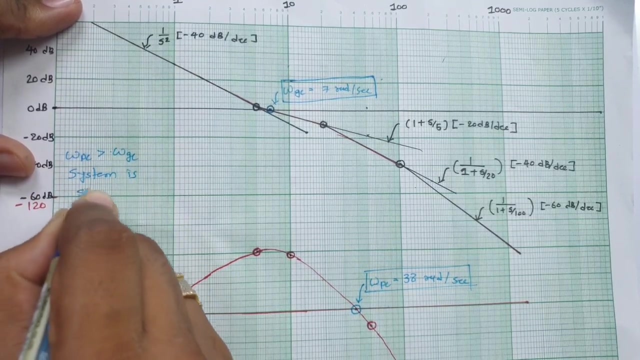 So it is 38.. So phase crossover frequency, that is 38 radian per second. So now we have two values Right Now here. one thing that one should note see: phase crossover frequency is greater than gain. crossover frequency means system is stable. 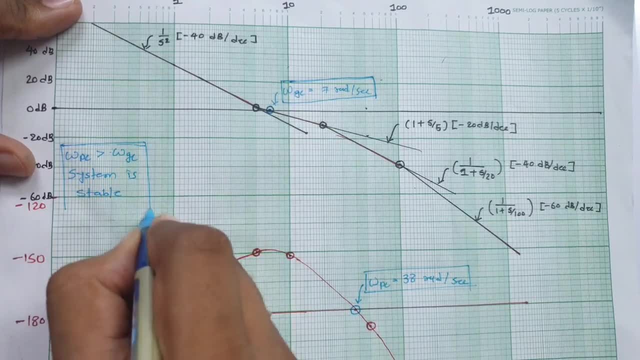 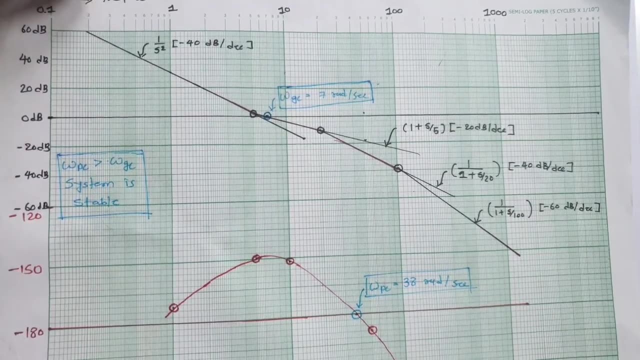 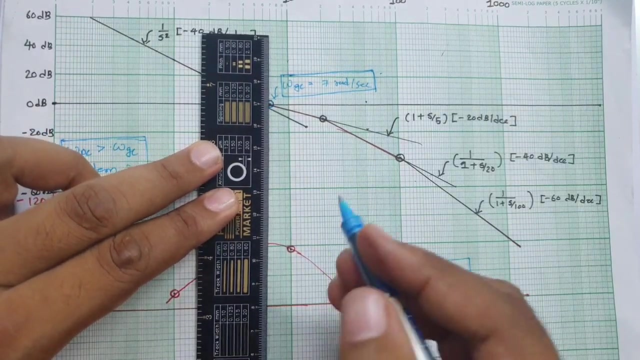 Here phase crossover frequency that is greater than gain crossover frequency. So we can say: system is stable. Now we need to identify gain margin, Right And phase margin for this table system. So all we need to do is we just need to stretch a line vertically. 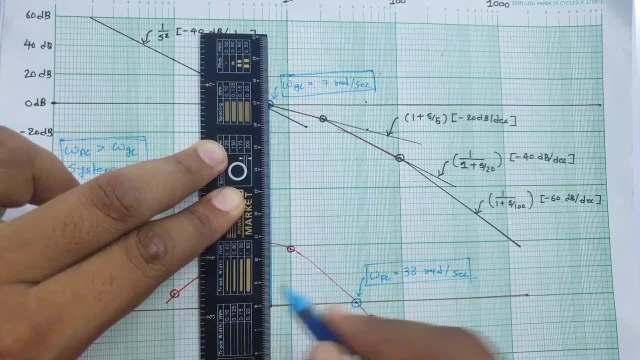 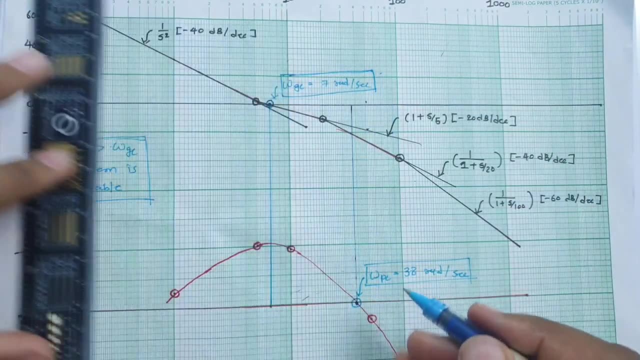 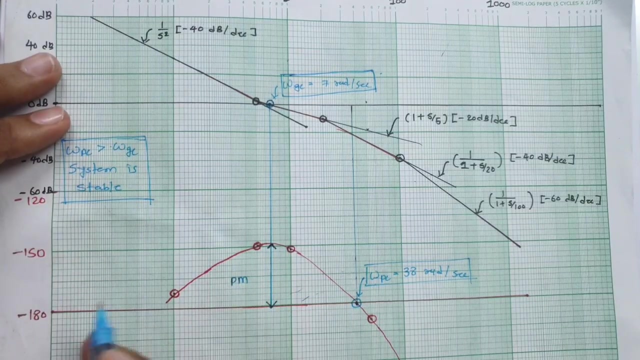 As you can see, for gain crossover frequency, I'm stretching it like this, And for phase crossover frequency, I'm stretching it like this vertically. So this is our phase margin And as per this you can say this is approximately 31.3.. 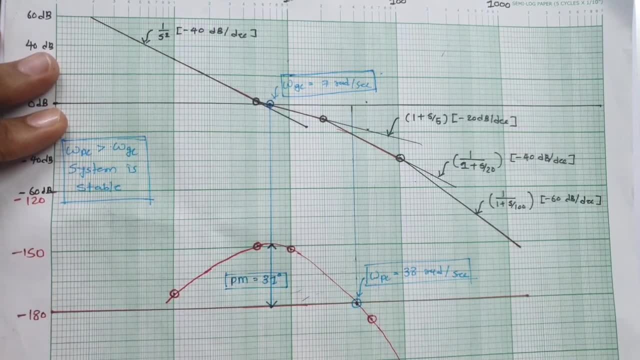 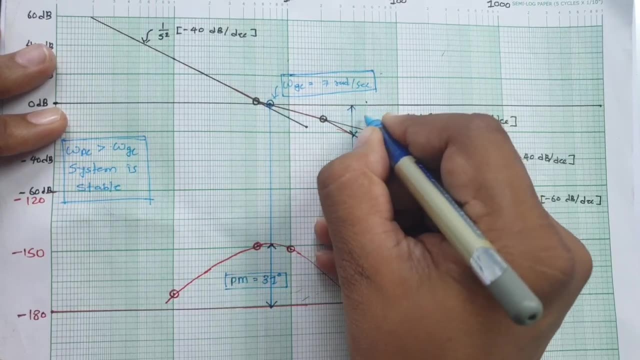 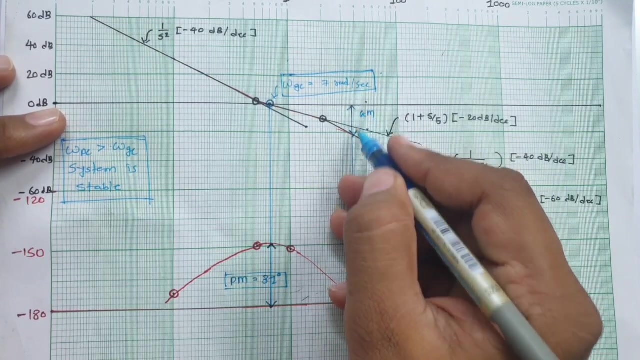 Right. So we have phase margin that is approximately 31 degree And if you stretch this line over here, you see, this is our gain margin And that is somewhat greater than 20.. One can say 21.. You see, Right. 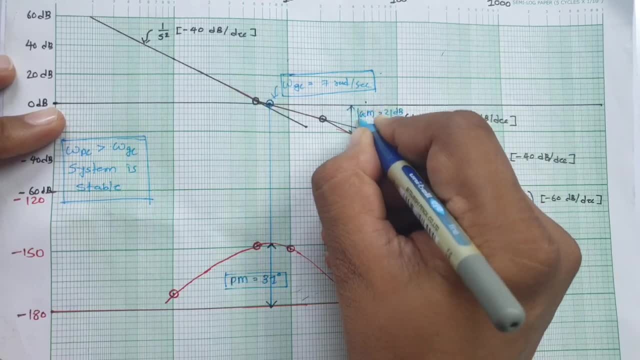 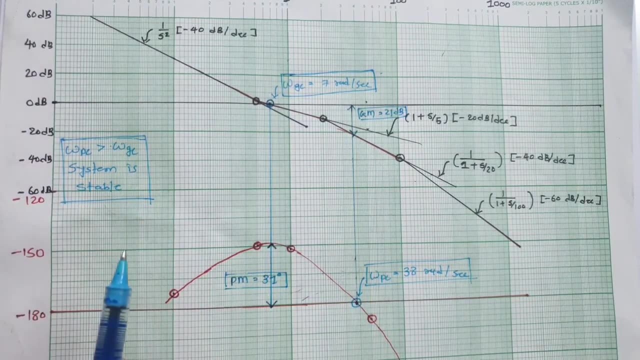 So I'm saying this is 21 dB. So here Phase crossover frequency is greater than gain crossover frequency. So system is stable And phase margin is 31 degree and gain margin is 21 dB. This is how we can identify Bode plot, step by step. 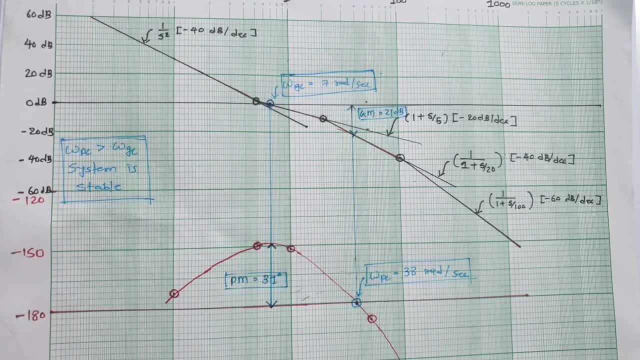 I hope you have understood this Now. if you have any query, you just place that in comment. Definitely I'll try to get back to you based on your queries. Thank you so much for watching this video.